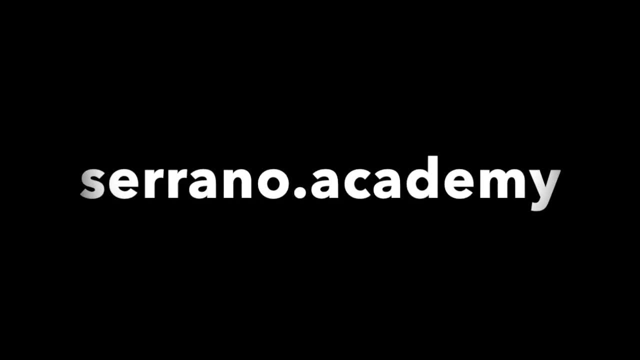 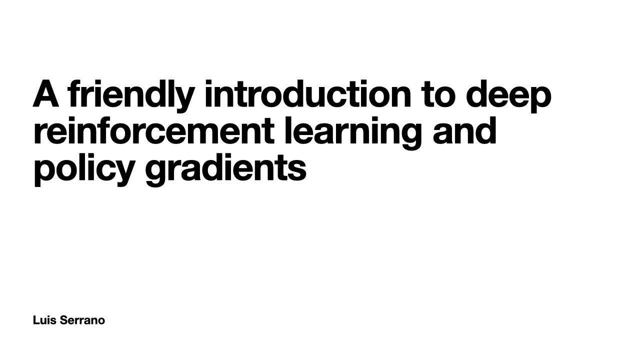 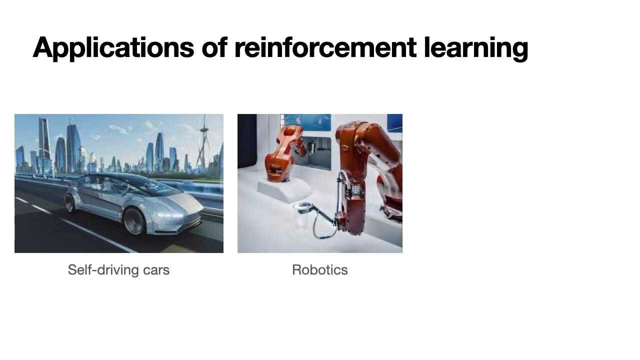 Hello, I'm Luis Serrano and this is a friendly introduction to deep reinforcement learning and policy gradients. Reinforcement learning has great applications in many cutting-edge fields, such as self-driving cars, robotics and even winning at complicated games like Go, Chess and Atari games. The difference between reinforcement learning and the more 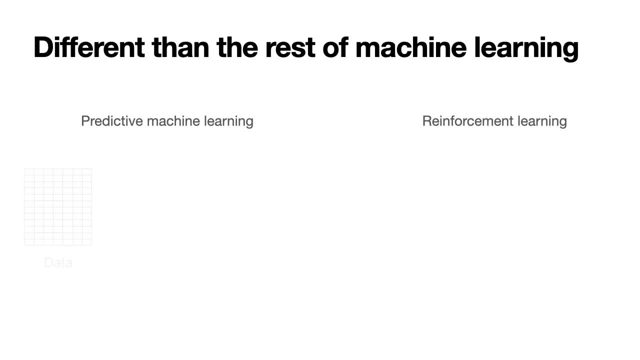 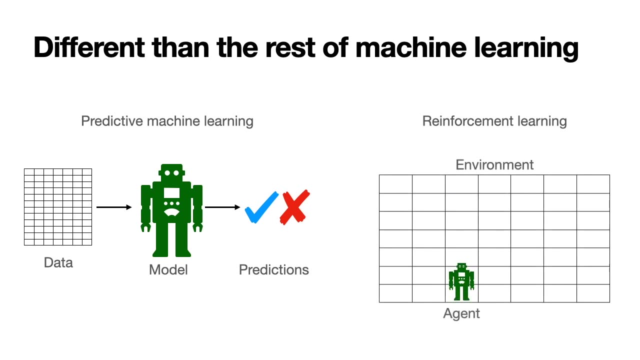 common predictive machine learning is that in predictive machine learning we have a lot of data, which is used to train a model, and then the model is used to make predictions or answer questions. In reinforcement learning we have no data. we only have an environment and an agent that lives in that environment. The agent moves around, collecting rewards. 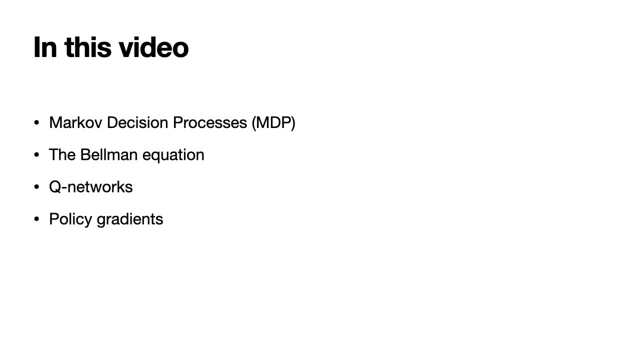 and punishments and creates the data as it goes. In this video we'll learn several important reinforcement learning concepts. The first one is a Markov Decision Process, or MDP. Then we learn the Bellman Equation, which is one of the building blocks in reinforcement learning. 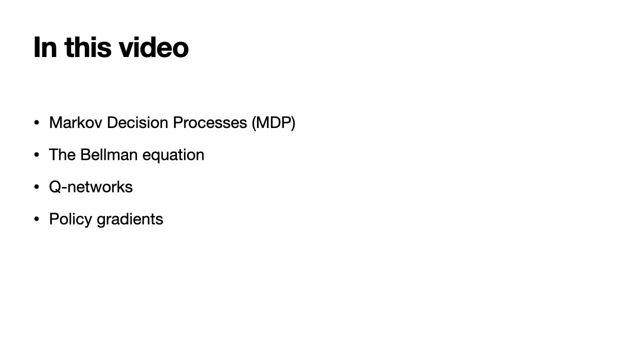 Then we learn how neural networks can help us with reinforcement learning when the problem is too big, as we'll see in Q-Networks and Policy Gradients. Alright, let's begin. The first example of reinforcement learning is a Markov Decision Process, or MDP. To illustrate: 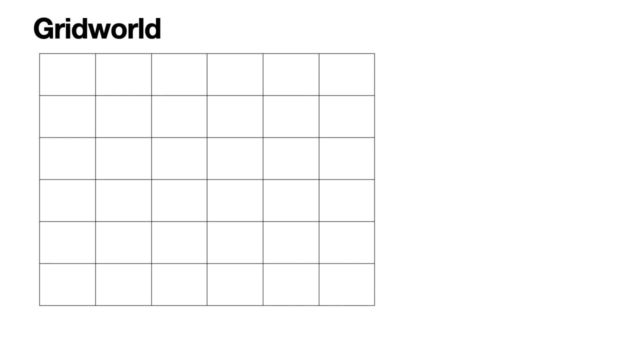 an MDP. we'll use a very common example: the grid world. In the grid world we have our universe, which is this grid, and our agent, which is this circle. over here And in this universe we have some very special squares. for example, over here we have a lot of money. 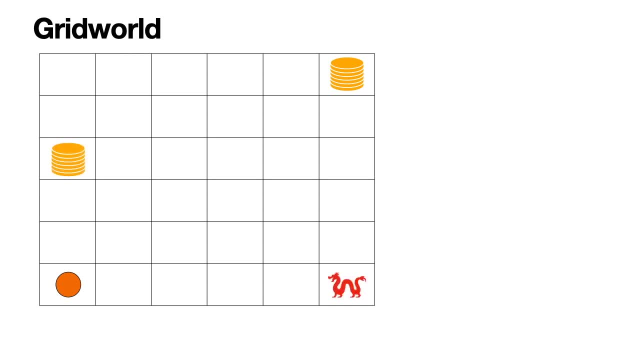 then some money over here too. and here we have a dragon that eats you if you fall into that square. Since we want to make it a game with points, we will add some points to each square. This one gives you 5 points, this one gives you 4. if you land them, then and? 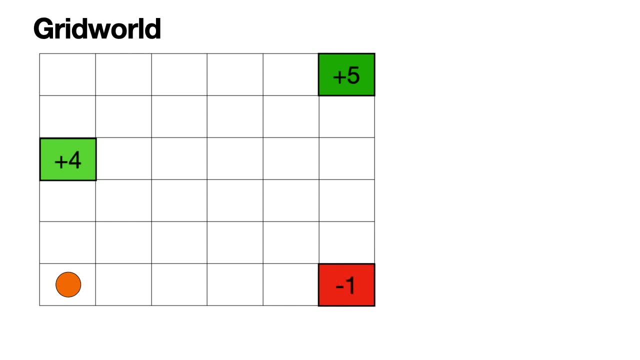 this one gives you minus 1.. All these are terminal states, meaning that when the agent falls on them, the game will end and the agent ends up with the points collected on that square. We also have some barriers that the agent can't pass through, so if it walks, 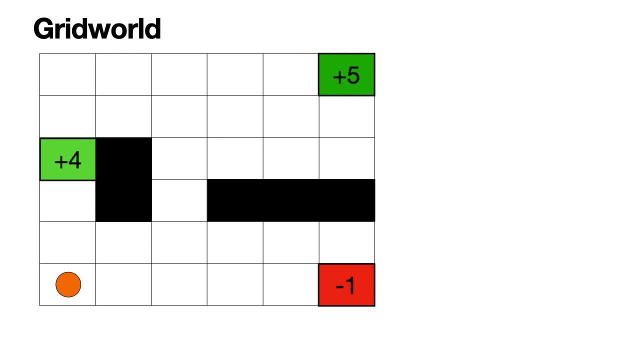 into them. it simply stays in the same place, And the point of the game is that the agent walks around the universe, always moving to an adjacent square, collecting rewards or punishments. Over here it landed in a plus 4, so it collects a plus 4.. Now let's play it again. Here it. 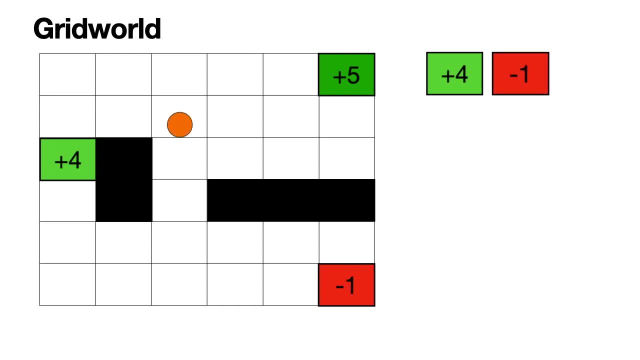 lands into the minus 1,, so it collects a minus 1, and so on. It doesn't need to start in the bottom left, it can start anywhere. Now the point of reinforcement learning is to teach the agent how to do as best as possible. 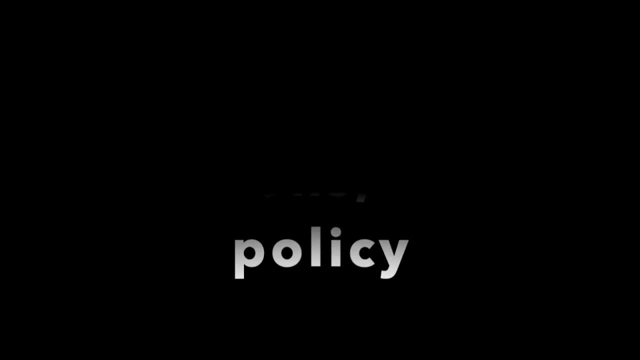 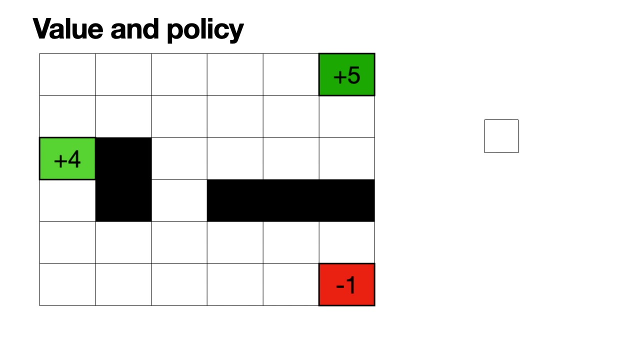 in this game, and that's what we'll see next. So, in order to come up with strategies, let's look at this square over here and let's say that these four other squares are its neighbors. Each square is called a state. We also have 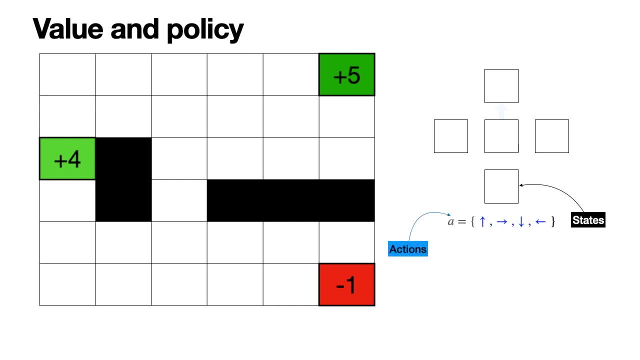 four possible actions, which are going up, left, down and right. And here's the thing. imagine that we gain 4 points by landing in the square on the right, 1 point for the square on top, minus 3 for the one on the left and 2 for the one on the bottom. These 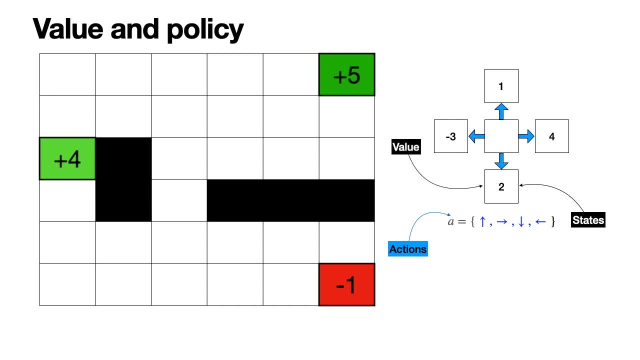 are the values corresponding to the states. Now, in this case, what is the best strategy for our agent? if what we're trying is to maximize the number of points, Clearly it is to go to the right and gain 4 points. This is summarized in this equation called the Bellman equation. 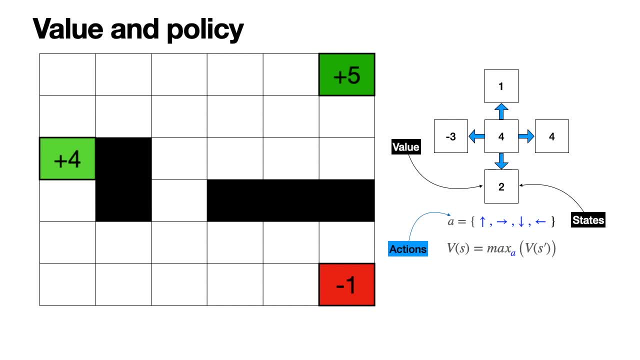 which is the main equation of the system. So the first equation is the Bellman equation, which is the main equation of the system. The second equation is the Bellman equation, which is the main equation of the system. It says that the value of the state S is the 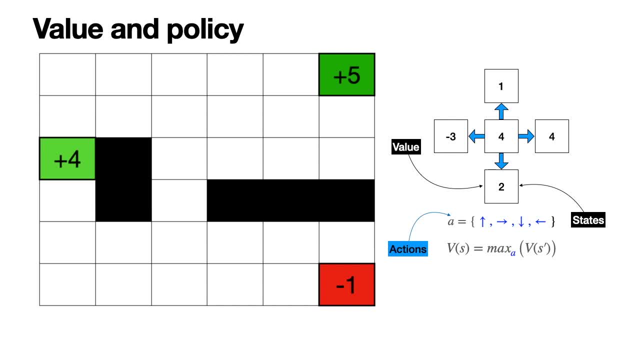 maximum of the values of its four neighbors, or the neighbor states that one obtains by applying any of the possible actions. And this is simply because the agent can walk to the best neighbor and obtain those points. So the value of the state is the maximum number. 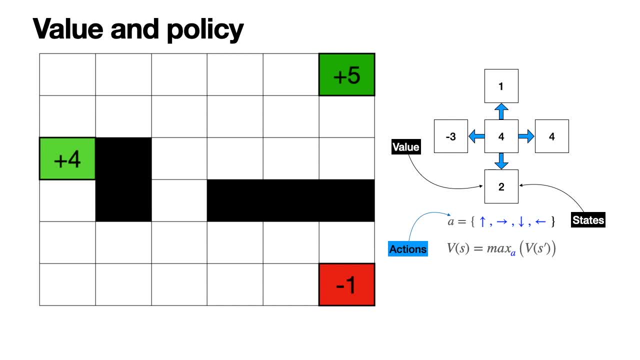 of points that one can obtain, going from that state and making the best possible decision. The best possible decision is called a policy, which we'll talk about in a minute, But for now let's focus on the value. For most of the states on the left, we don't know the value, We only know it at the terminal. 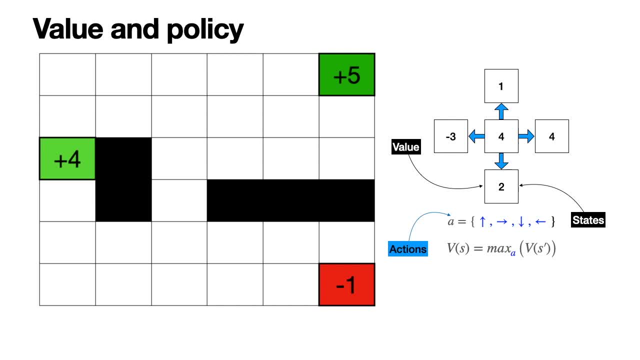 states which are plus 5,, plus 4, and minus 1.. But notice that for the neighbors of 5, we also know the value now, and it's 5, because we can figure it out using the Bellman equation. 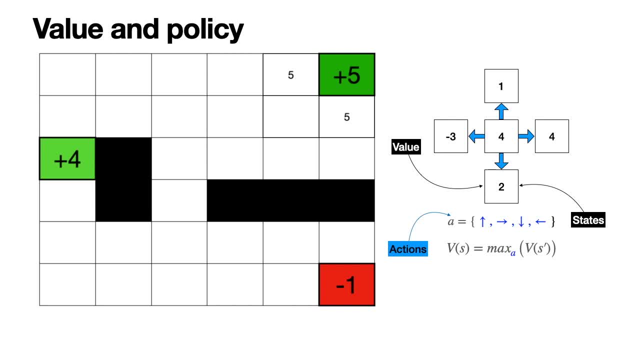 because, as they are neighbors of a 5, then the 5 is the maximum you can do by going among all your neighbors, And we can propagate this to the neighbors as well, and so on. And if you notice carefully, you'll see that the value of the state S is the maximum number. 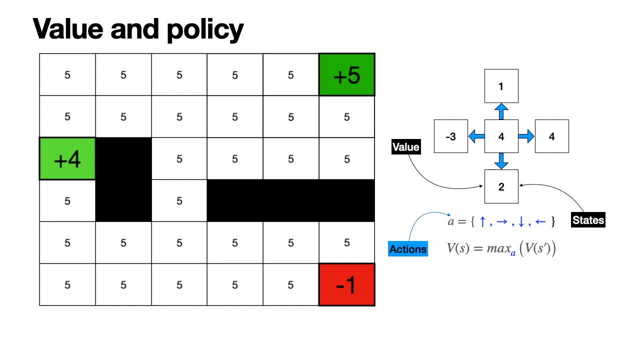 of points that one obtains by applying any of the possible actions. So the value of the state S is 5, because from every state you can walk some way towards the plus 5 and claim your 5 points, and that's the best decision. 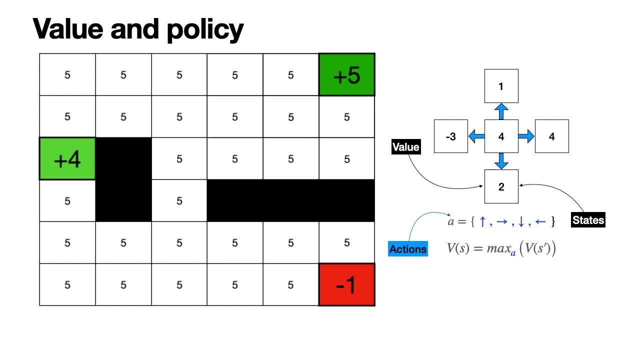 Now let's talk about the best decision. Let's talk about the policy. The policy is the set of instructions to always take the agent in the best possible path with respect to gaining points. I like to imagine the policy as arrows in the floor, instructing the agent where to 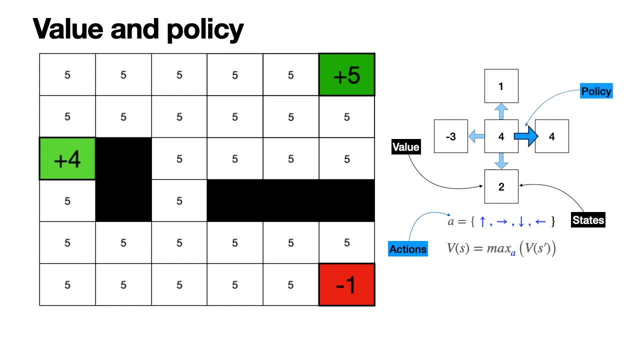 fall. And as for the policy, well, as long as we make sure that we don't fall into the plus 4 and we don't fall into the minus 1 and we get to the plus 5, we're good. So this: 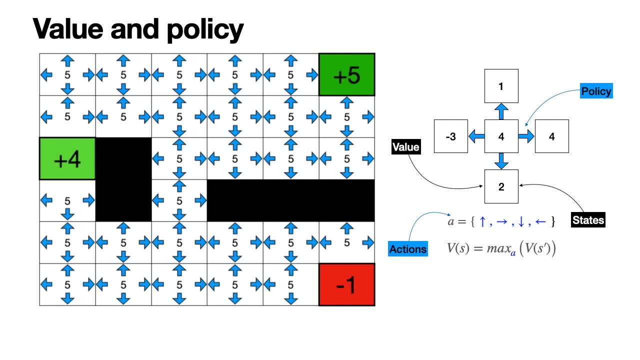 is a decent policy, because if we always take one of the available arrows, we'll get to the 5, we'll never be stuck at the minus 1 or the plus 4.. However, this seems like it's not very efficient. Here's a slightly better one that's not going to make us crash into. 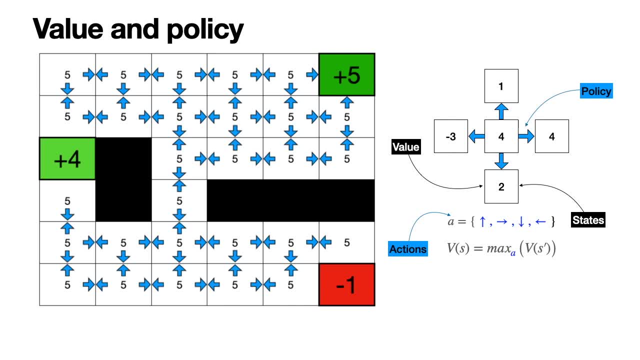 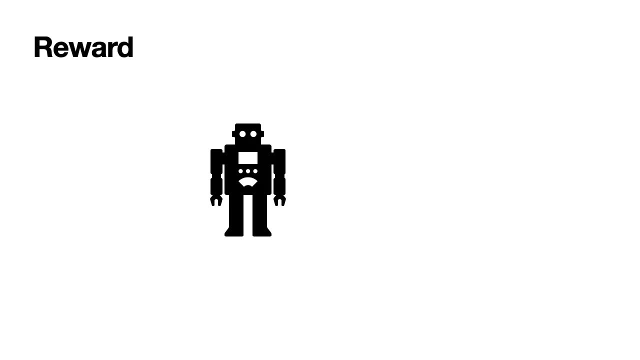 the walls, But it's still not ideal. Let's introduce some modifications that will make sure that the agent can get to the 5 faster, or to wherever it has to get, instead of wandering around forever. The idea is to slightly punish the agent for walking around aimlessly, and for that we introduce 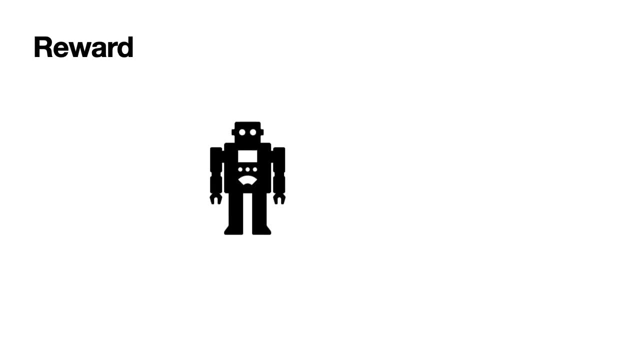 the reward. The reward, which can be positive or negative, is an amount of points the agent picks up when taking any step. In this case it is negative if we can imagine that the agent getting tired or losing energy or gasoline. In any case, it is expensive for the agent. 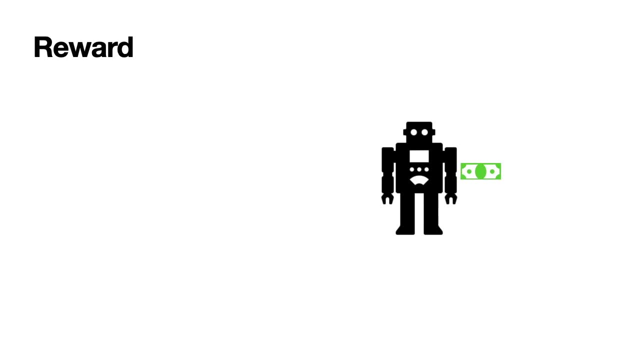 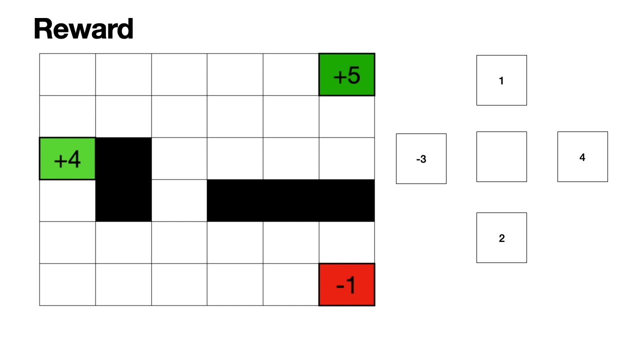 to take one step, so the agent will want to minimize the number of steps needed to reach a terminal state. Let's say that we have the same neighbors as before and each step costs the agent one point. Therefore, the reward is negative one. 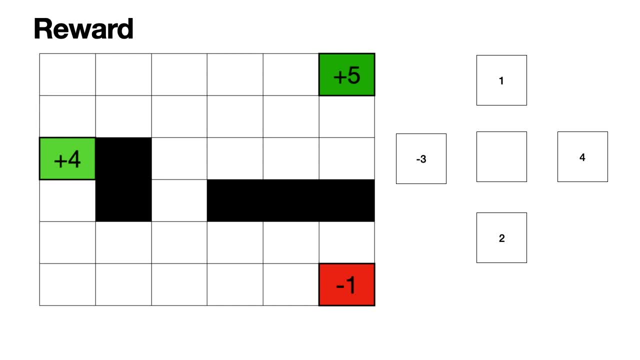 Now let's revisit our equation for the value. So if the agent picks up four points by moving to the right, since the reward is negative one, then now the value is gonna be four minus one, And we can do the same calculation if we go up. 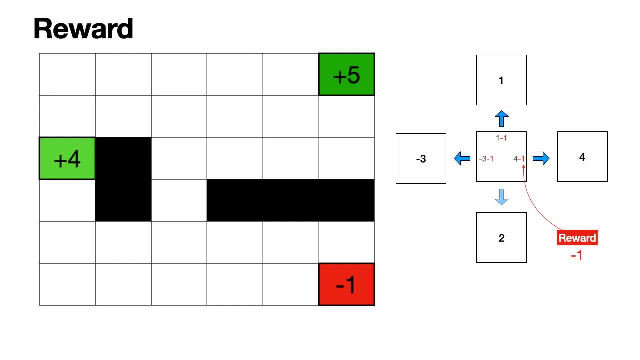 one minus one. if we go to the left, minus three minus one, and if we go down, two minus one And again, the best strategy is moving to the right, which is the one with the highest value. So now our value is four minus one. 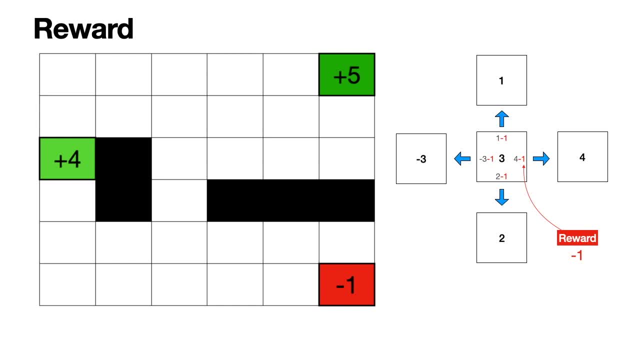 which is the reward, which is three. Therefore, our Bellman equation changes a little bit. It's still like before, where the value of a state is equal to the maximum, over all its neighbors, of the value of the neighbor, except that now we have to add the reward. 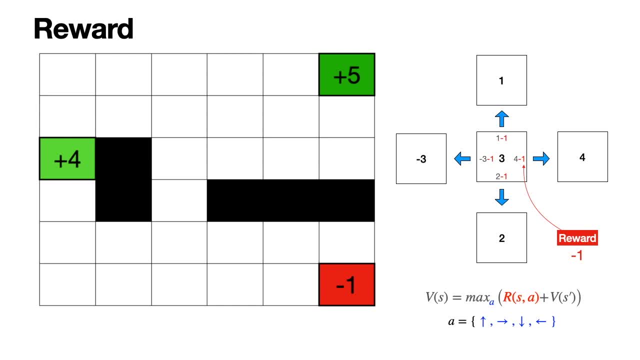 which is negative one. And now, using this Bellman equation, we can start to propagate the values from the plus five. For example, its neighbors are now gonna have a four, because we need to subtract the reward If the neighbors of these fours are gonna have threes. 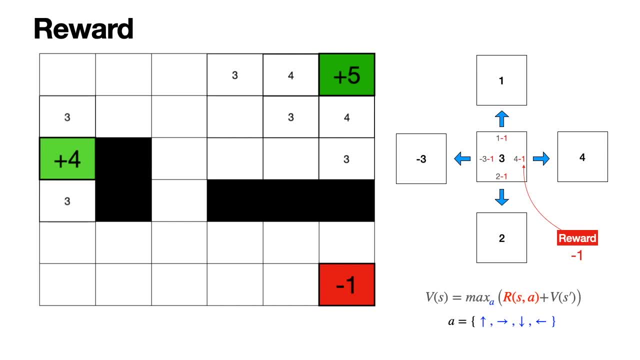 now let's look at the neighbors of the plus four: They're gonna have threes and their neighbors are gonna have twos, and the neighbors of the minus one are gonna have minus twos. And we can continue in this way, filling out every box. 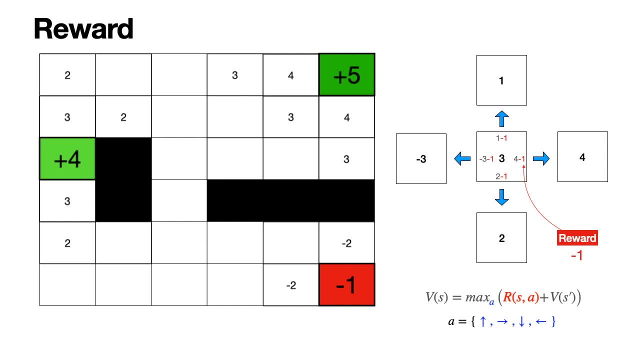 And sometimes we may need to go back to a box and revisit it, because the values on the neighbors will change. But if we continue doing this, I encourage you to give it a try. We get these values. Each value is the maximum of points you can obtain. 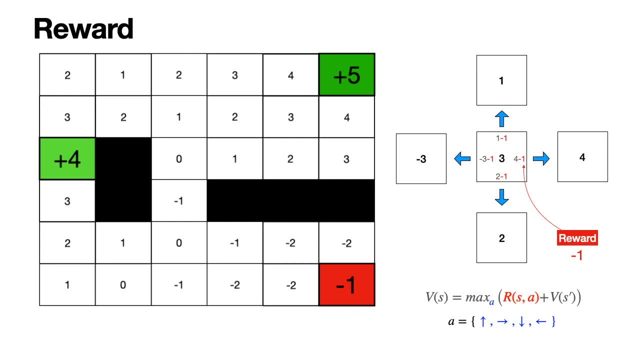 if you walk in the best possible way, And that best possible way is given by the policy. The policy is simply a bunch of arrows that, from each square, they point to the neighbor that has the highest value. Notice that sometimes there are ties and two neighbors have the same highest value. 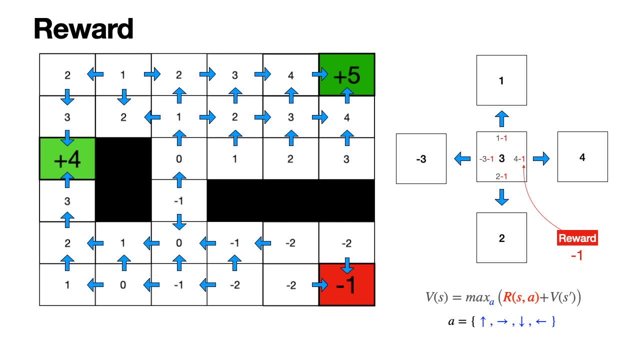 You simply draw all the arrows that correspond And when the agent is walking around, the agent can pick randomly which one to take among those winning arrows. Now check out something interesting. Imagine that your agent is here and you're wondering what to do. 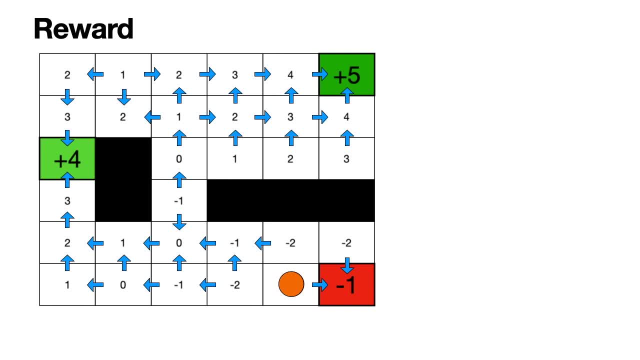 The policy says you can't go into the minus one. but why? Well, the reason is that it's much more expensive to go to the five or to the four. Yes, you do gain some points, but you lose more in the process of walking. 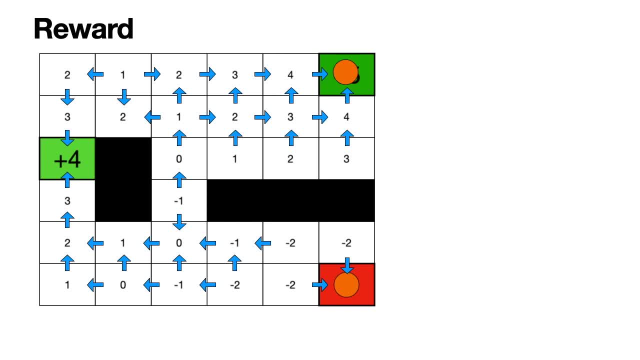 The way I like to see it is: imagine if you really have to go to the bathroom when you're in a rush and there's a really nice bathroom 10 kilometers away, but it's too far for you and you'd rather just go to the closest one. 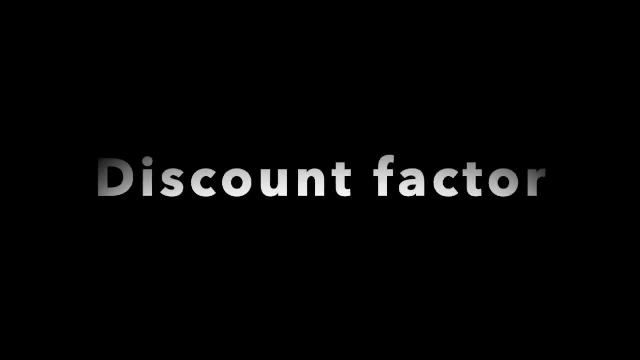 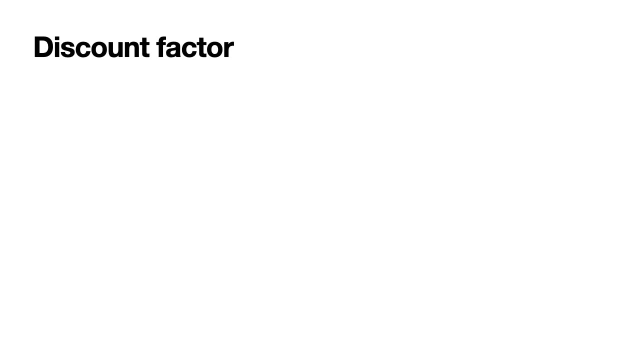 even if it's just an okay bathroom. Another way to get the agent to speed up is to use a discount factor. The philosophy behind the discount factor is that a dollar today is worth more than a dollar tomorrow, and is worth even more than a dollar in two days. 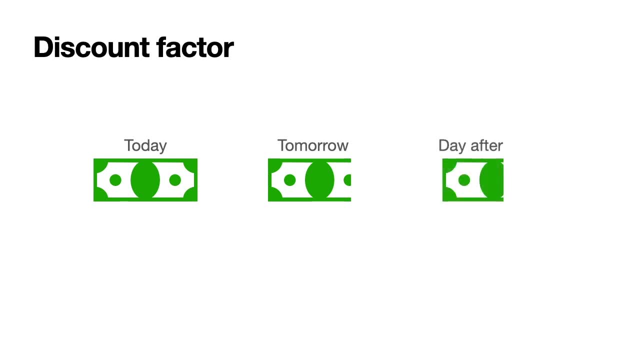 This is because it's better to have the money now and to have a promise that you'll get the money later. For example, if a dollar today is worth one, a dollar tomorrow can be worth, for example, 90 cents, and a dollar the day after would be 81 cents. 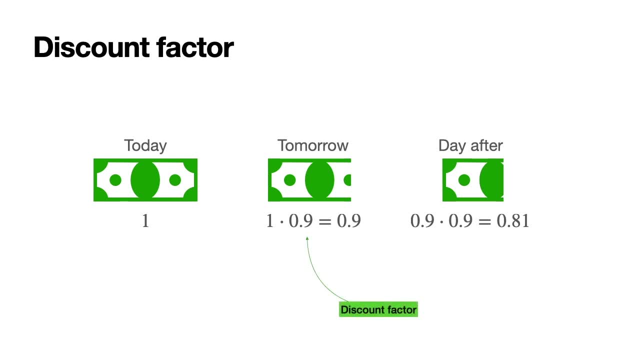 which is 0.9 times 0.9.. So in this case, the discount factor is 0.9, and for every day that passes we multiply the value of our money times 0.9, and that's what it's worth. 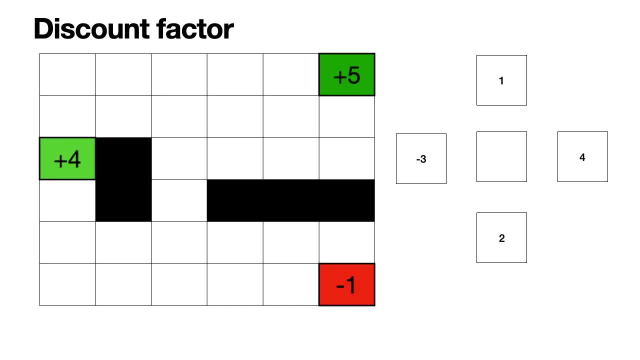 if we were gonna have it tomorrow instead of today. Thus, if we were to walk into a state, for example, with a four, then the current value is gonna be four times 0.9, which is 3.6.. 0.9 is the discount factor. 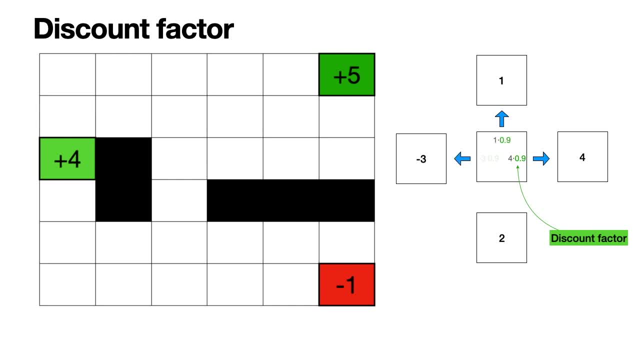 The same happens if we go to the top, to the left and to the bottom, And so our Bellman equation changes again, because now it says that the value of a state is the maximum, over all its neighbors, over all the states, I can obtain by applying the actions. 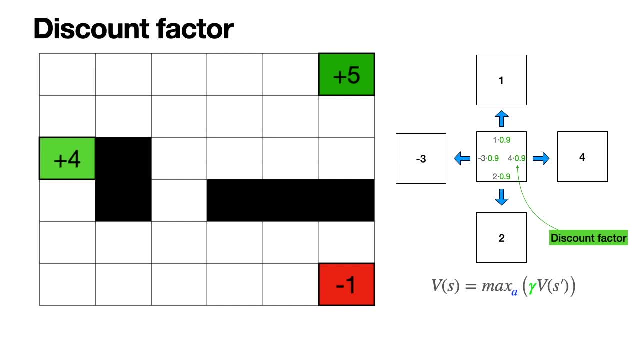 of the discount factor, gamma times the value of that new state. And so again, the best strategy is to go to the right, because we are going to gain four times 0.9, which is 3.6.. And again we can start propagating. 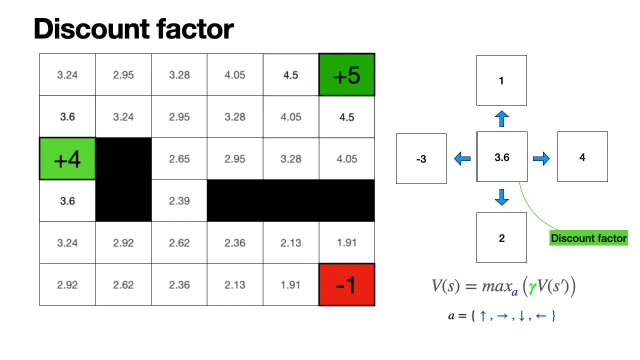 the values from the five and from the four, et cetera, et cetera, And again I encourage you to work this out. These are the values I got for the values at each state. And again, the policy is obtained by drawing arrows. 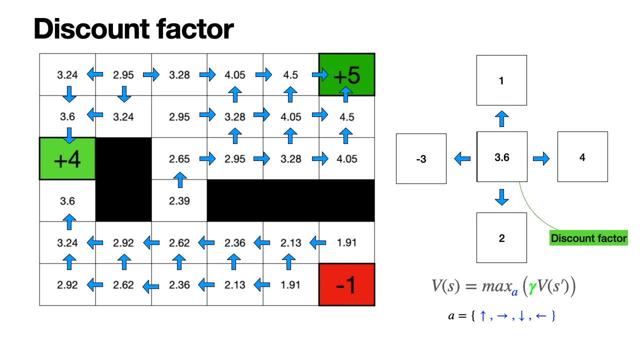 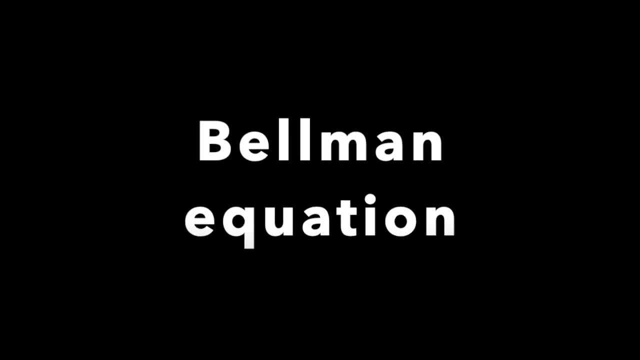 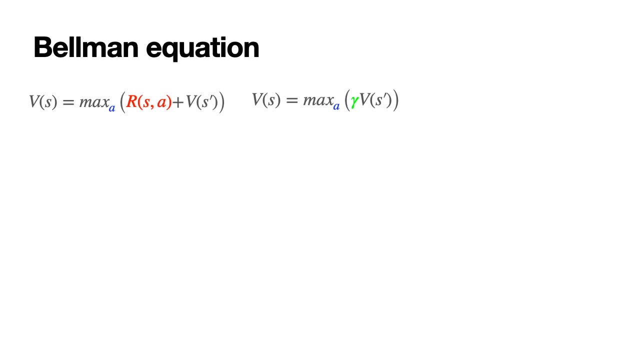 that point from every state to the neighboring state with the highest possible value around them. We've seen two equations so far, namely one with a reward and one with a discount factor. The Bellman equation is a combination of these two. In this one we have that: the value of a state. 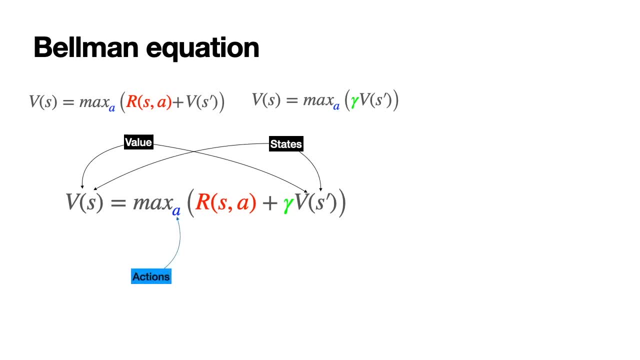 is the maximum number over all the possible actions one can take of the reward, plus the discount factor times the value of the neighboring states. In our case we have that the actions are the four cardinal directions, The reward is negative one and the discount factor is 0.9.. 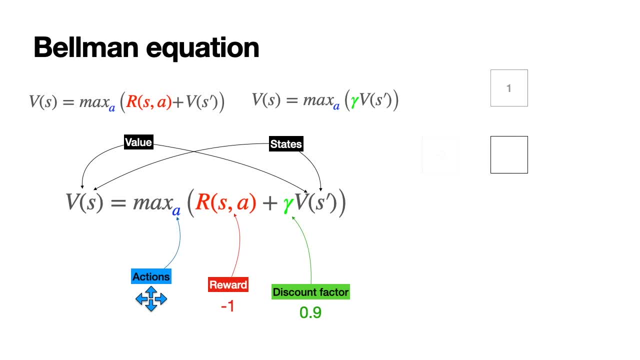 Therefore, in our ongoing example, where these are the values of the neighbors, we know that we have to walk to the right, which is the highest value, And the value of our new box is gonna be four times the discount factor of 0.9,. 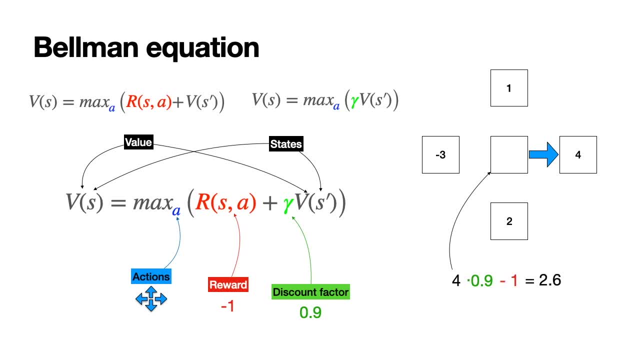 plus the reward, which is minus one, and that's gonna be 2.6.. Now, in some cases in the literature you will find the Bellman equation with an extra term which is negative one, and that's gonna be 2.6.. 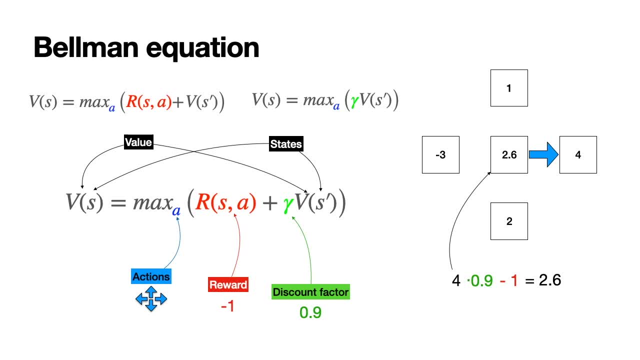 Now, in some cases in the literature, you will find the Bellman equation with an extra term, which is a probability. That is a probability that the agent may not take the action you have instructed it, It may disobey or it may make a mistake. 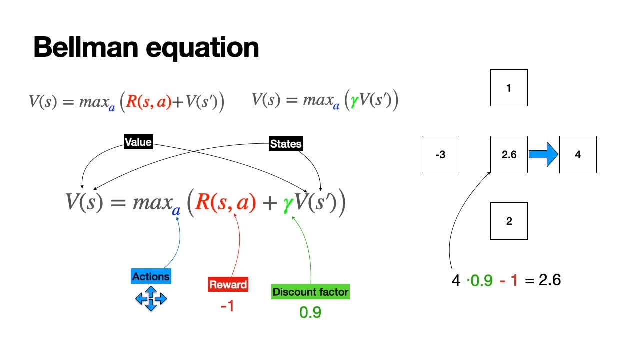 or fall to the side with certain probabilities. This complicates the Bellman equation, but we're not gonna focus on this because today we're gonna focus on neural networks, So this may be the subject of a later video. Now for this video. in order to keep the math clean. 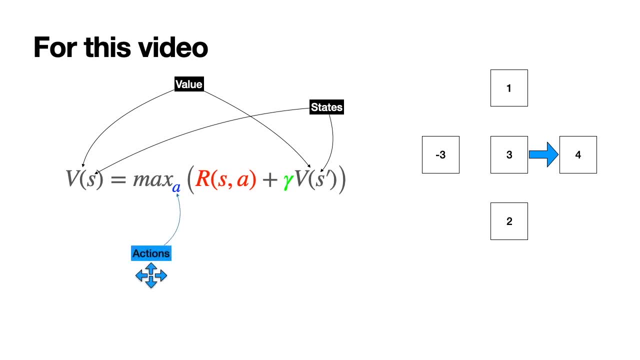 and not have so many decimals. then we're going to consider again the actions, the four cardinal directions. the reward- negative one- but the discount factor: we're gonna take it to be one, which means there's really no discount factor. 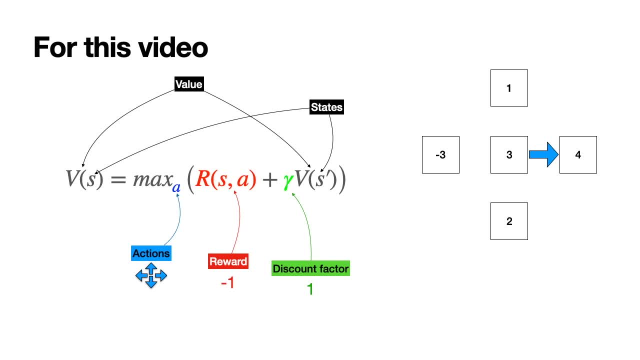 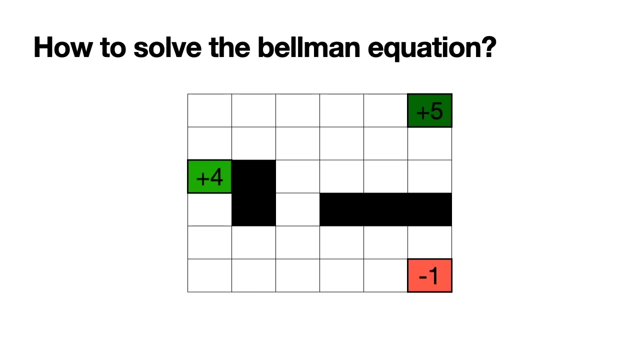 A dollar today is worth as much as a dollar tomorrow. But I encourage you to follow the math that we do with any other discount factor and work out the numbers. Now that we've seen the Bellman equation, the question is: how do we solve it? 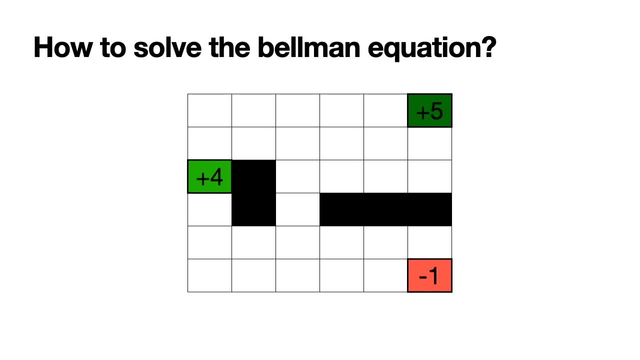 In other words, how do we find the values for all the states? And the answer is iterating. We start by picking random states and using the Bellman equation to calculate their value. Now, for most of them, there's no value for the neighbors. 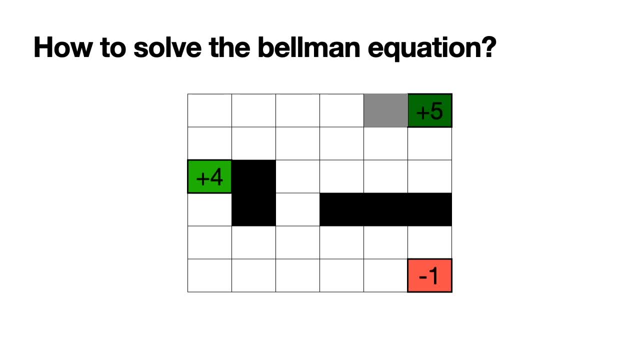 so we can't do anything. But one day we'll bump into this box over here, And since one of the neighbors is five, then the value for this one is gonna be a four, as the reward is negative one and the discount factor is one. 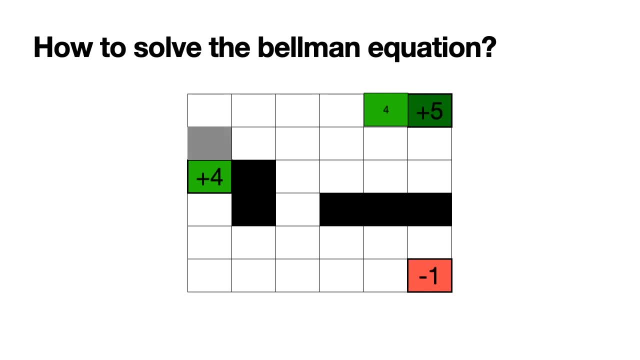 Then we keep walking and one day we'll land here, And for this one the value is three, based on the Bellman equation. And then later we bump into this one and the value is negative two. And we can continue picking random boxes. 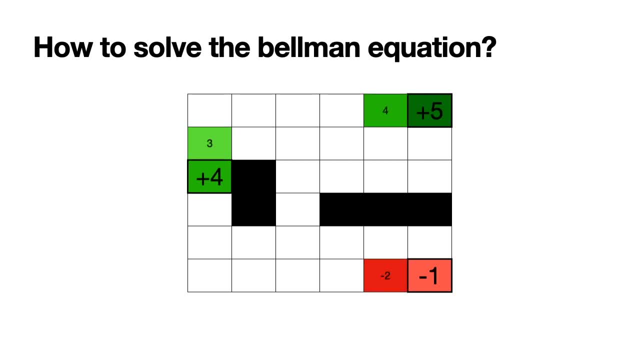 and using the Bellman equation. Now what happens? Let me show you how we can get into an ambiguity. If we pick this box, then the value is two by the Bellman equation. If we pick this box, then it's one. 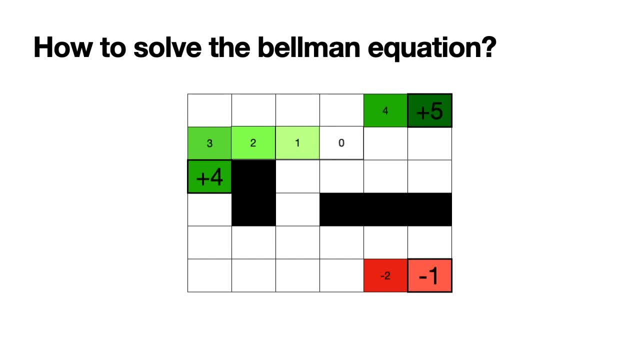 And if we pick this box, then it's zero, because the biggest neighbor is a one, And once we pick this box, well, the biggest neighbor is a four, so the value is three, And now we've messed up the one for the bottom. 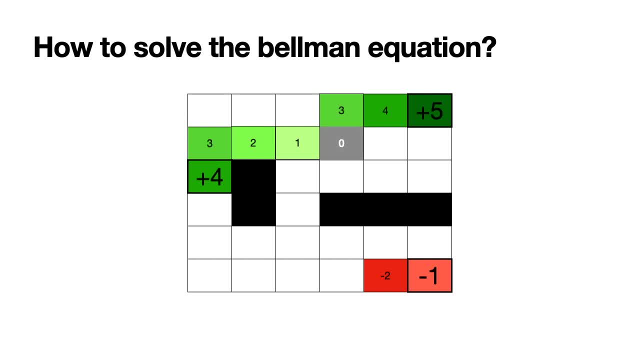 because that one is wrong, Doesn't matter. We keep picking boxes and maybe one day we'll get to this box and we'll fix it, because the maximum value of the neighbors is three, so therefore this value is two. So if we go over all the boxes many, many times, 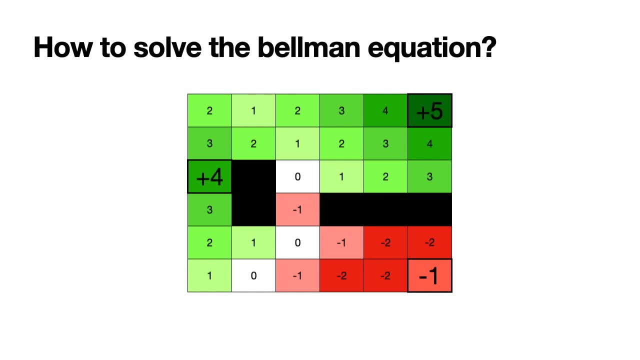 eventually we'll converge and we'll get something like this, which is the correct value for every state, where the Bellman equation is always satisfied, And if we want to come up with a policy, all we have to do is draw arrows that go from each box. 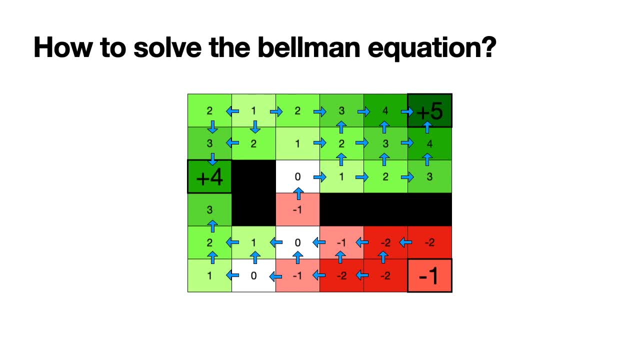 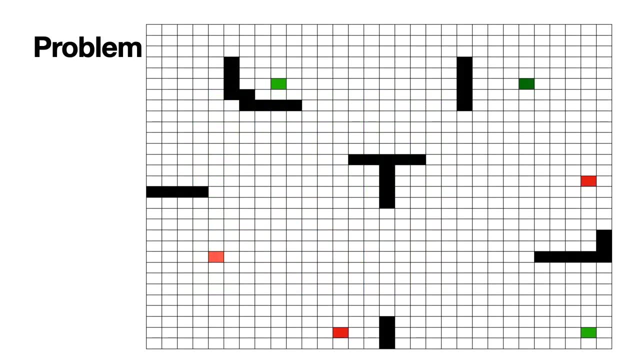 to the box of highest value among its neighbors. So all is well in this small example, but what if we have a much bigger example? The algorithm says you have to visit every box not only once, but several times until the values start converging, and that's impossible to do. 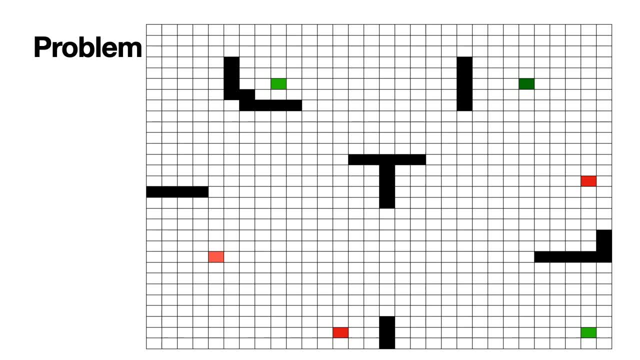 when you have a very, very large universe with millions of states and actions, et cetera, It's very expensive to go over all of them over and over and over. so what can we do? Well, this is where neural networks come to a rescue. 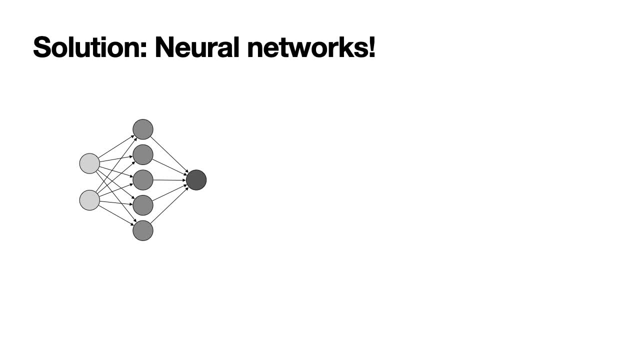 Neural networks will come in two ways: one of them for calculating the value, which is called a value network or a Q network, and the other one for calculating the policy, which is called a policy network. This video assumes a basic familiarity with neural networks. 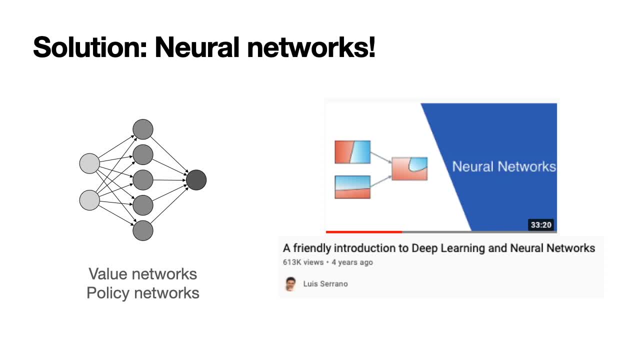 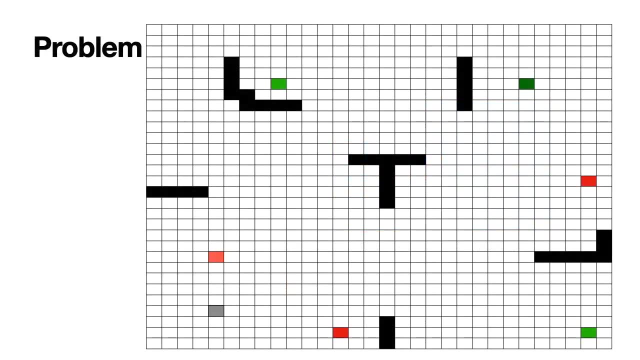 If you'd like to catch up on these, then I also recommend this video on my channel, where I introduce them, and the link is in the comments, And this way we won't actually have to go over every state several times to learn the value of the policy. 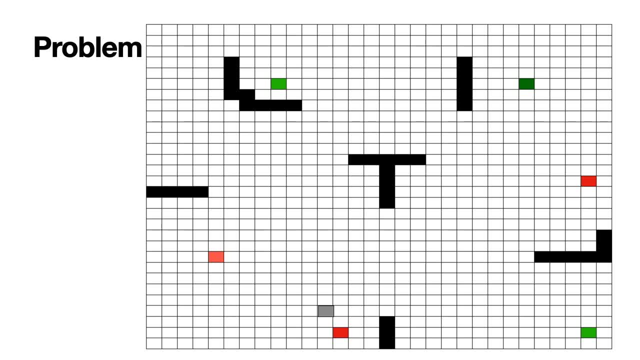 we simply have to let our agent wander, and the neural network will be smart enough to pick up information from the places that this agent manages to visit and propagate them to the entire grid, And this is not only good for saving time, but also for saving space. 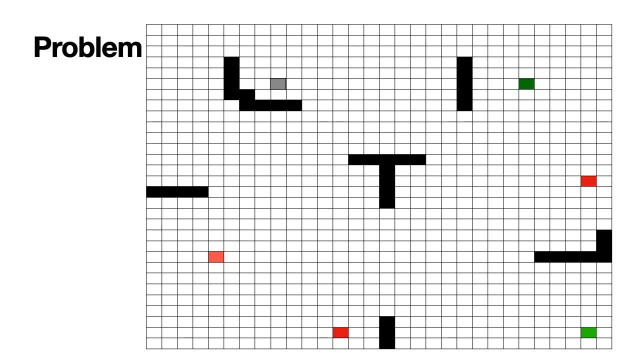 Imagine how much space we need to store all the values or policies of the states on the right And for some examples, for example, to win the game of Go. there are more states than the number of atoms in the known universe, so we can't even store them. 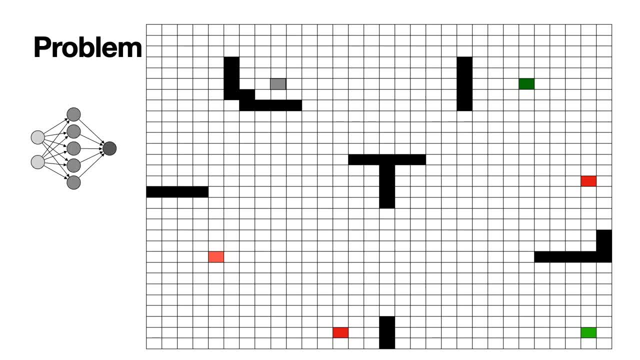 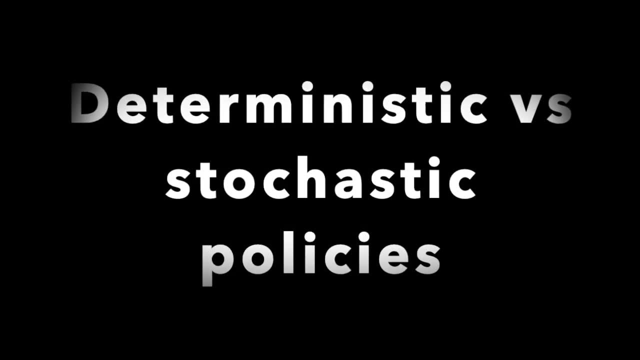 A neural network, however, may have much less parameters, so we can actually store all that information, or at least a very good approximation to it, And that's why we use neural networks to solve reinforcement learning problems. But before we get to neural networks, 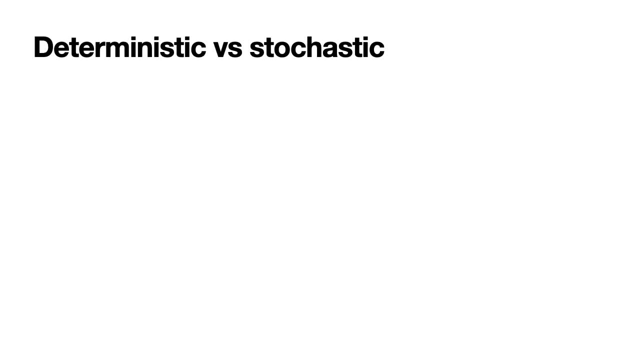 let me tell you a bit about deterministic and stochastic policies. Imagine that we have this scenario where we have an agent and some money at the right, but a lot more money on top And we walked around the space enough to figure out a policy that can find the money at the right. 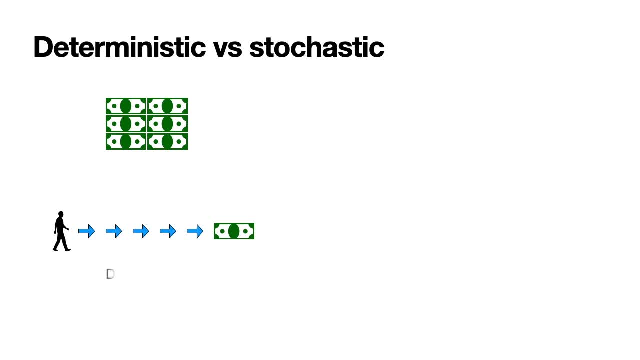 but we haven't yet found the money on the top, And deterministic policy is one that says always move in this direction. Such a policy will for sure get the bill at the right, but could potentially miss the money on top. Can we fix this? 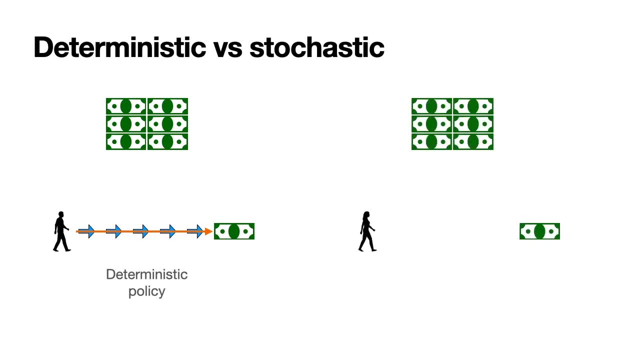 So the way we fix this is with a stochastic policy, which means a policy that goes in the right direction but it's also less strict and gives wiggle room for exploration. So a stochastic policy will say yes, with a large probability you should walk. 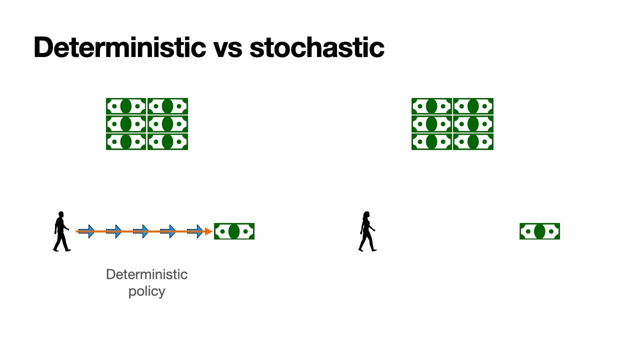 towards the bill that we've already found, but with some probability you should still be able to walk in the other direction so that you can explore the space, And if we have that at every point in the space, then the agent will be able to walk. 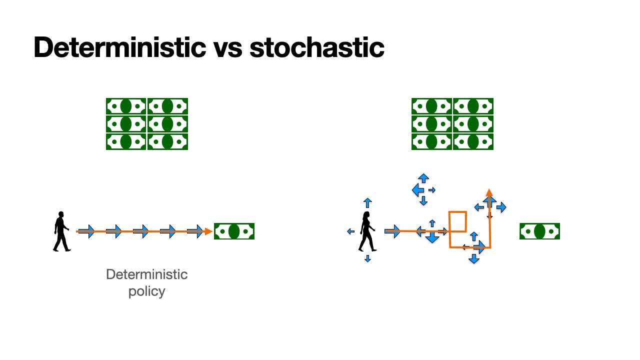 and very likely end up at the bill, but with some probability, explore the rest of the space and be able to find all the money on top. So that is a stochastic policy. A stochastic policy is better, is better for training and therefore we will use it to train these neural networks. 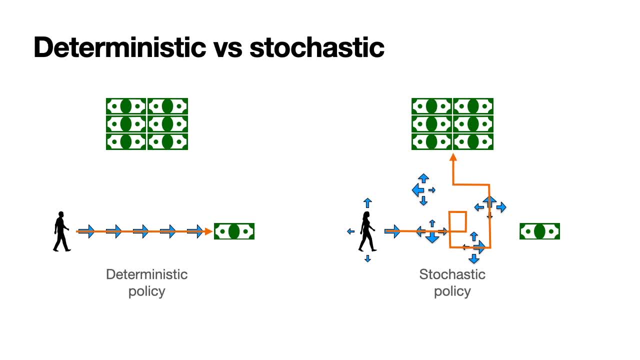 This is also called explore-exploit, where exploit means you try to use the policy to gain as much as possible and explore means you also give yourself wiggle room to look around the space, even if you don't get the best reward every time. 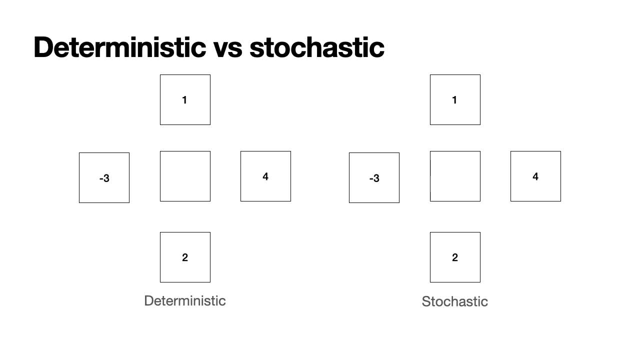 but you still be able to find new things. A deterministic policy looks like the one on the left, where it indicates that the agent should go to the right to find the best value. The policy indicates to the agent to move to the right with probability of one. 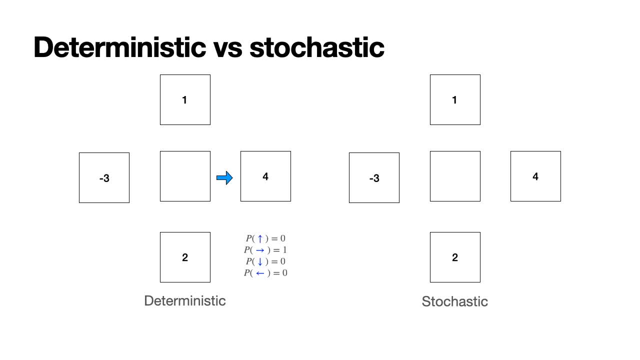 and to move to the other directions, with probability of zero. A stochastic policy, in contrast, would tell the agent to strongly go towards the right, but it still give the other states a chance based on the reward it obtains, For example, the stochastic policy on the right. 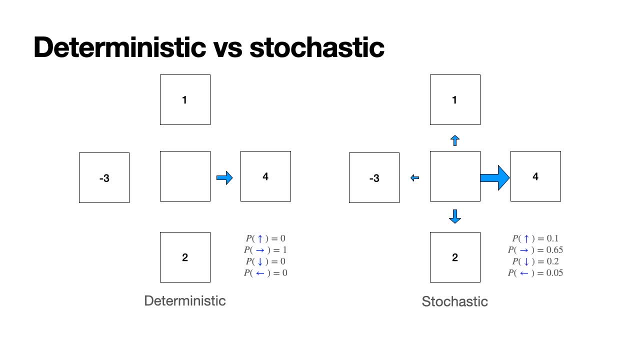 will give the state towards the right the most priority because the value is the highest there, and the state, the state of moving to the left the lowest priority because the score is the lowest, but it still make them non-zero, so you can walk around. 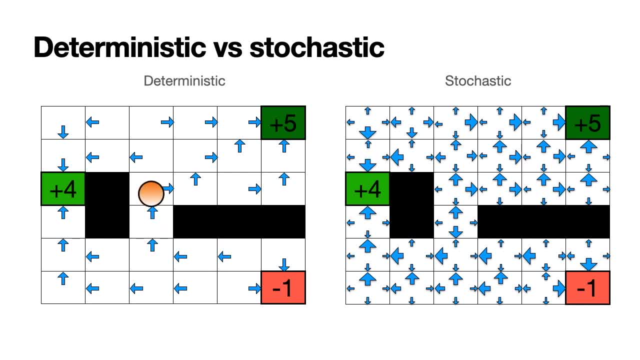 In a deterministic policy, the agent will only have one way to go, as in the left, whereas in a stochastic policy, the agent will be able to walk around the space, even if it doesn't get the best reward every time, but it still is able to explore the space. 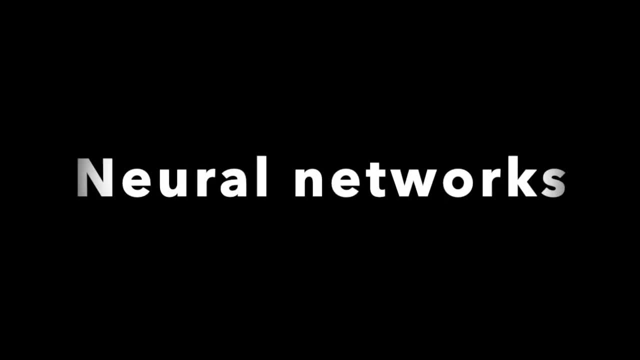 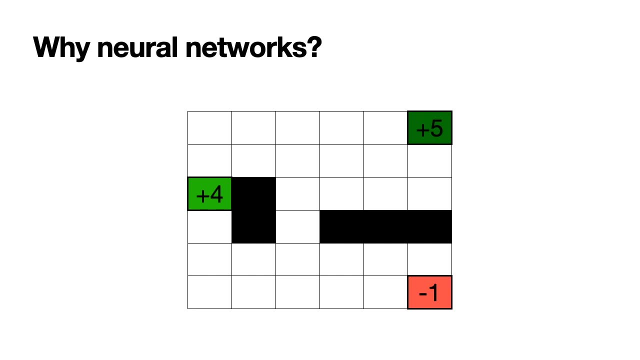 and potentially find better values. Now we finally get to the cool part: neural networks. As I mentioned before, having an agent try to visit all the states repeatedly is simply way too expensive, and we need to gather information by only visiting a few of the states. 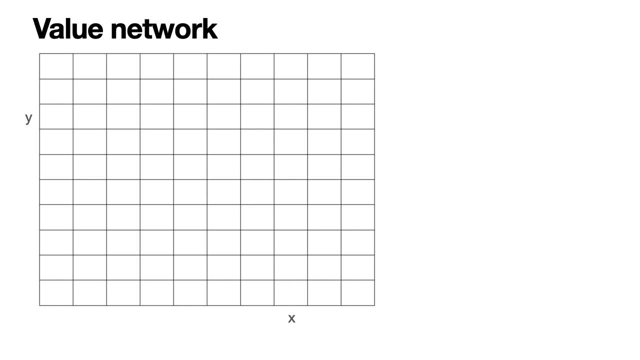 This is where a neural network can help. A neural network can say: hey, if the value of this state is large, then that means the values of the states close to it should also be fairly large, because a state influences its neighbors. Same thing with a small value. 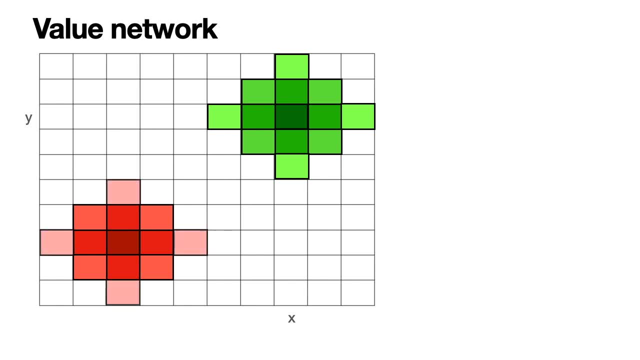 If the value here is small, then the values of the neighbors should also be small. A neural network can pick up that type of information. What we'll have is a neural network where the inputs are the coordinates of a point and the output is the score at that point. 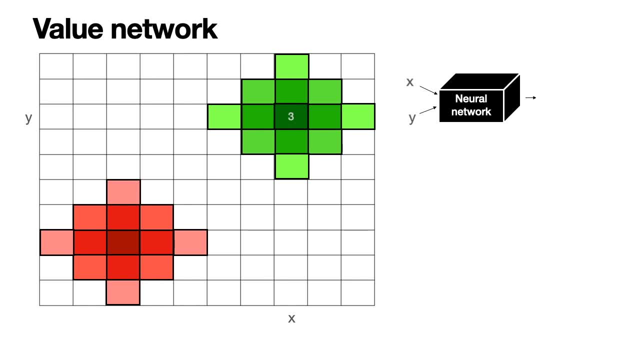 A neural network will make sure that closed states have closed values and that if we figure out the value of a state then we kind of know the values of its neighbors. And this one is a value network And the value network looks like this: 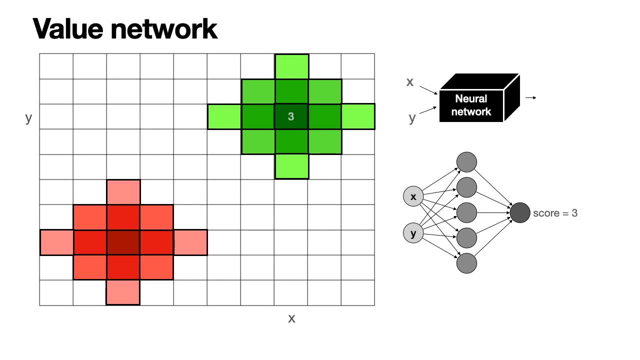 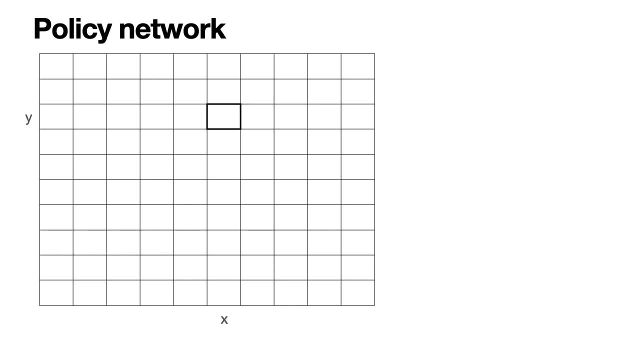 where, as I said, the input are the coordinates and the output is the score or the value at that state. We can also go even further and say: hey, let's not worry about the values, Let's worry about the policy right away. 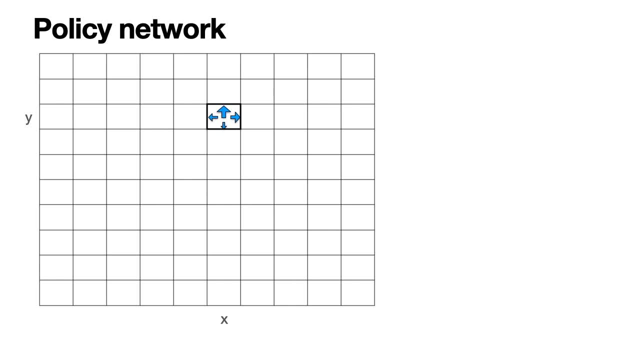 For the same reason as before, the policy at a certain state should be close to the policies of the states around it, because if at this point you should probably go up, then at the points around it you should also probably go up. So therefore, policies have the same behavior as states. 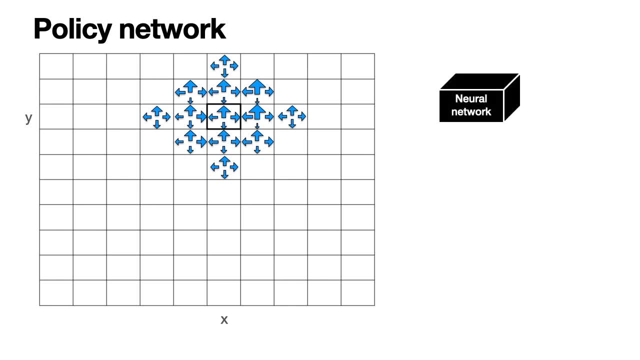 and we can model them with a neural network. This neural network again takes as inputs the coordinates of the points X and Y, and the output is the policy, which is four numbers that add to one, and these four numbers are: 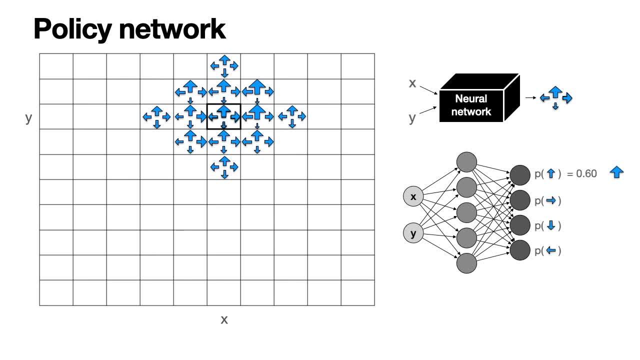 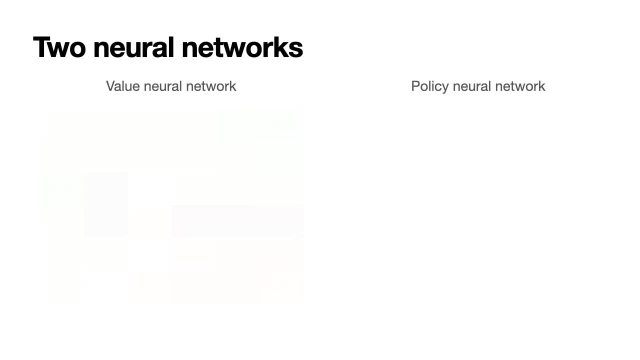 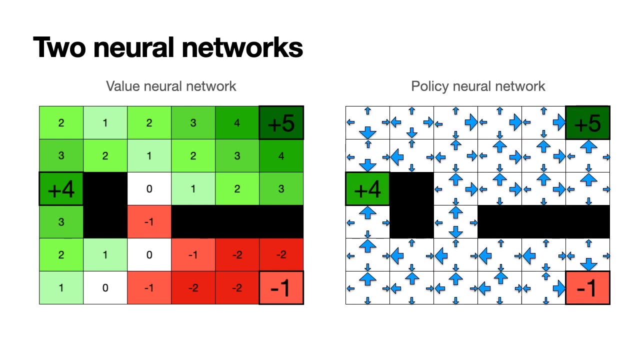 the probabilities of going up, right, down and left. So this is the policy neural network. In summary, we're gonna have the value neural network, which is the one that approximates the value at each state, and the policy neural network. 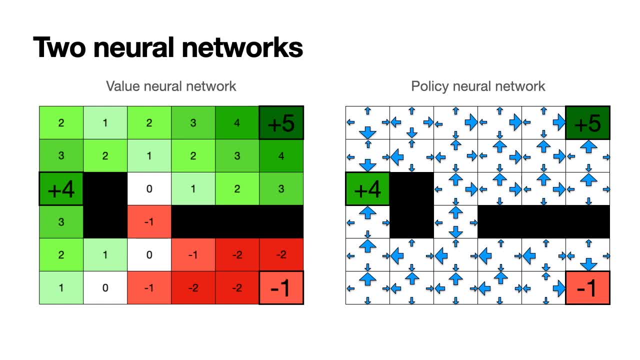 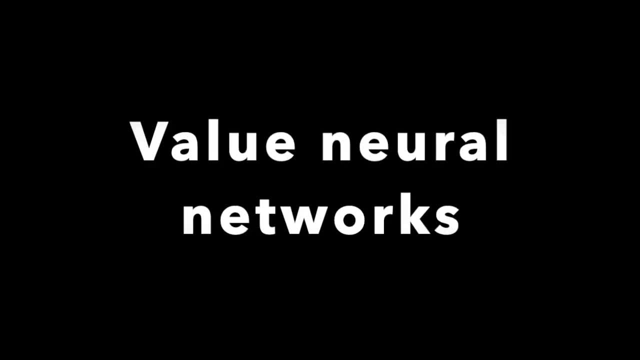 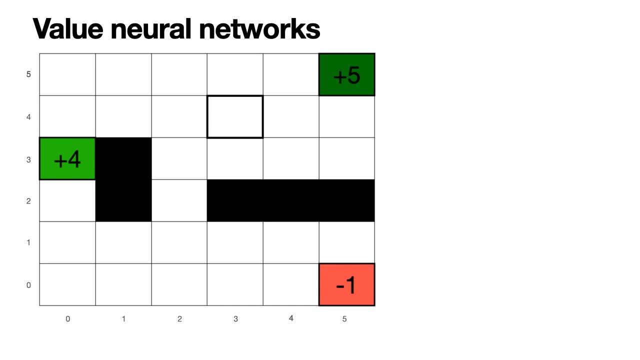 which is the one that approximates, at each state, the policy to take. Now we're gonna study both of them separately. First let's study value neural networks or Q networks. Again, what a value neural network does is from the values of a few states. 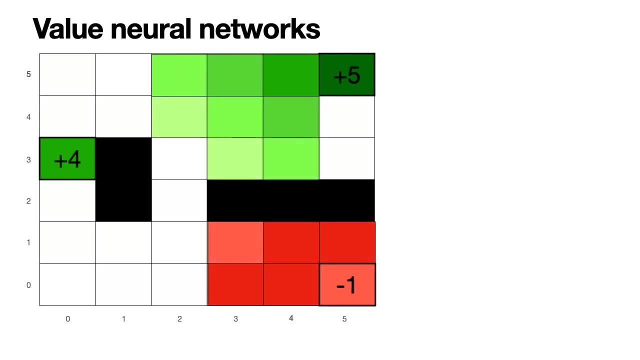 it propagates the values to the rest of the states And, in short, it takes as inputs the coordinates of the point corresponding to the state and the output is the value of the state. Now the question is: how do we train this? 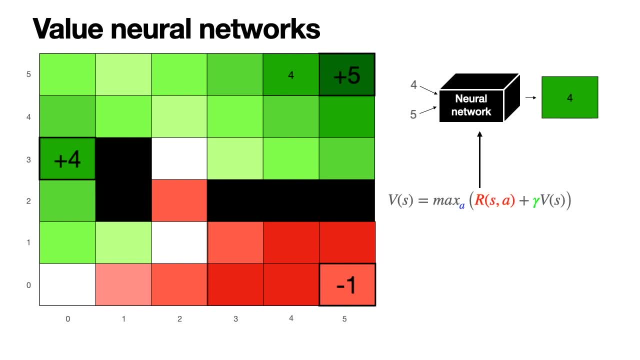 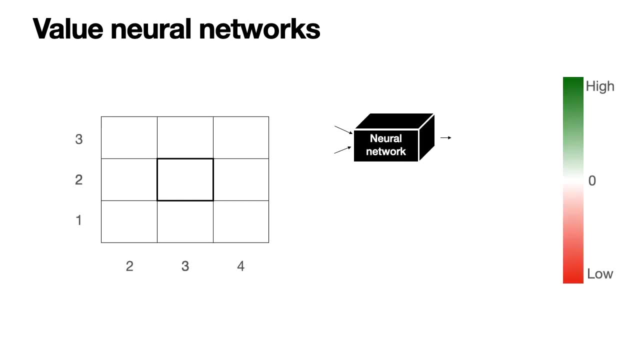 Well, we basically force them to satisfy the Bellman equation repeatedly, So we cook that into the error function. Let me show you how to do this. Imagine that we have a state corresponding to the box with coordinates two, three, And let's say that we have a randomly initialized 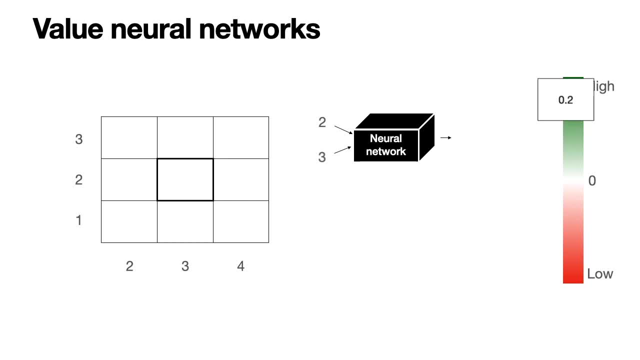 neural network which outputs a score of 0.2.. Now there's no reason for this one to be the actual value, because the neural network hasn't been trained, but we'll still use it And we'll use the values that it gives us at the neighbors. 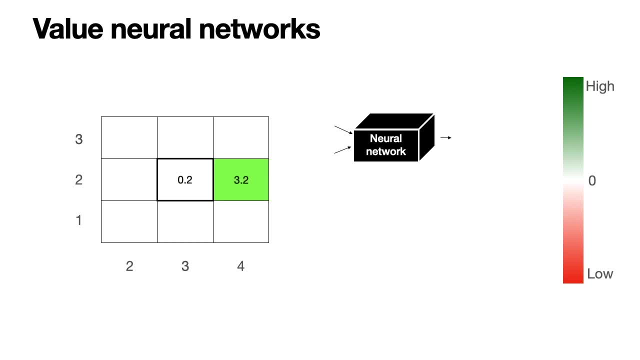 So the neighbor at the right gives us a 3.2,, the neighbor on top gives us a 1.3,, neighbor on the left gives us a minus 2.7, and the neighbor on the bottom gives us a 4.9.. 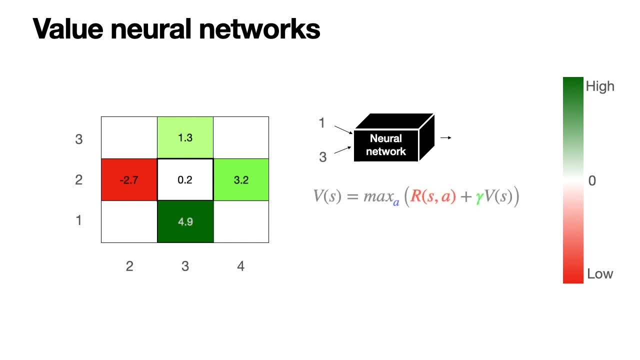 Now, these values clearly don't satisfy the Bellman equation. What would we have to do for them to satisfy the Bellman equation? Well, all we have to do is change the value in the middle. So recall that the Bellman equation is the maximum. 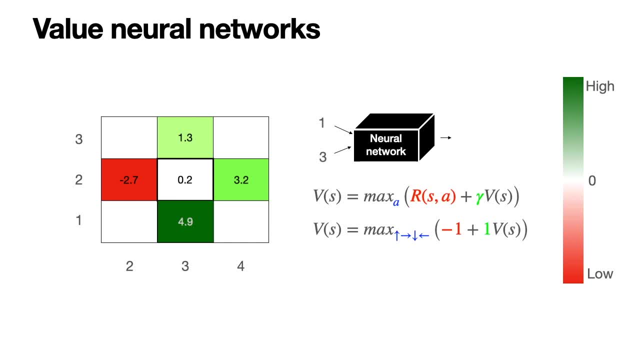 over all the actions, of minus one, which is a reward, plus V of S times one, which is the discounted value, the discount factor. So let's see what the box in the middle should have to satisfy the Bellman equation. Well, the neighboring states have values of 3.2,, 1.3,. 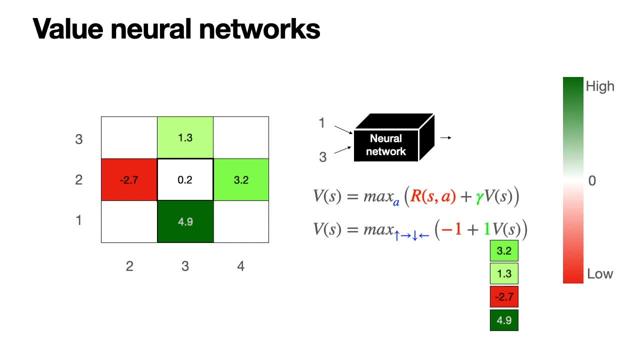 minus 2.7, and 4.9,, according to the neural network. We subtract one and we get these values 2.2, 0.3, minus 3.7, 3.9, and now we take the maximum. 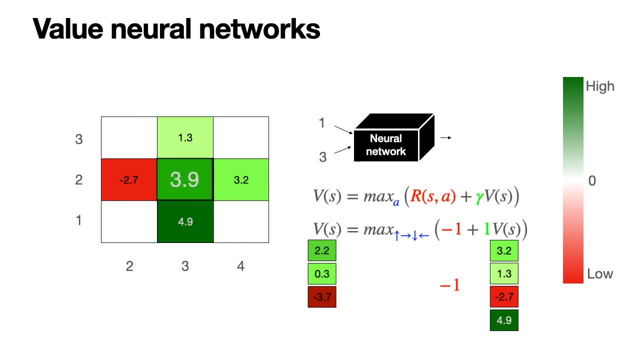 which is 3.9.. So we're gonna tell the neural network, you know what You need to make that value in the middle at 3.9.. And how do we tell it? Well, we add a data point to it. 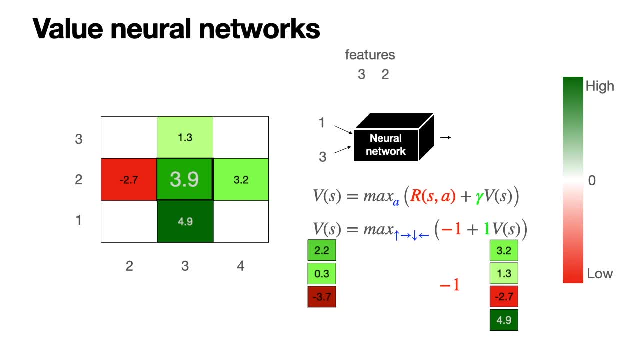 Data point has features three and two, the coordinates of the box and a label of 3.9.. And we say neural network. please take this data point and get yourself a little closer to outputting at 3.9 when I input a three and a two. 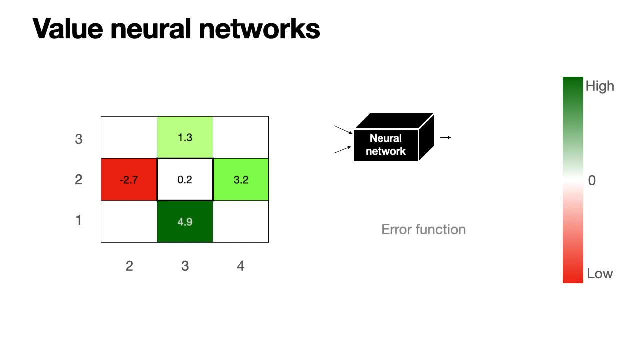 Now, if you like to think in terms of error functions, this is the error function. at this point. It's gonna be the square of the difference between the value given by the neural network and what the value should be according to the Bellman equation, with the values given by the neural network. 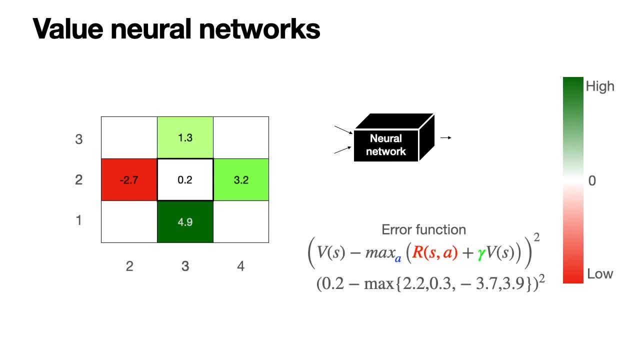 So it would be this over here: Now: if we take a gradient, descent step in that direction to improve the value of the box 3.2, we're not gonna get the 3.9 that we want, because these are tiny steps and we may get something. 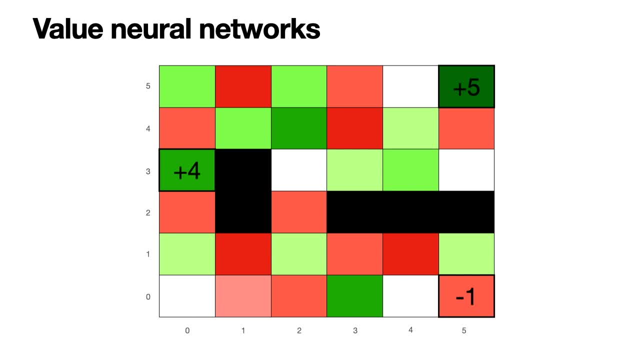 like a 0.45.. Now I don't blame you if this process looks a little unbelievable because you are using the Bellman equation with values that the same neural network gives you. But think that eventually, at some point, you will reach the points that are close. 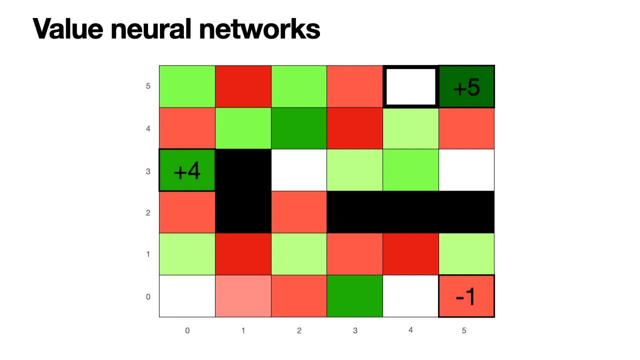 to the terminal states and they will help you change the values in a more accurate way, And they will also change the values of all the neural network And if you do this for a long time, I hope you believe with me that this will result. 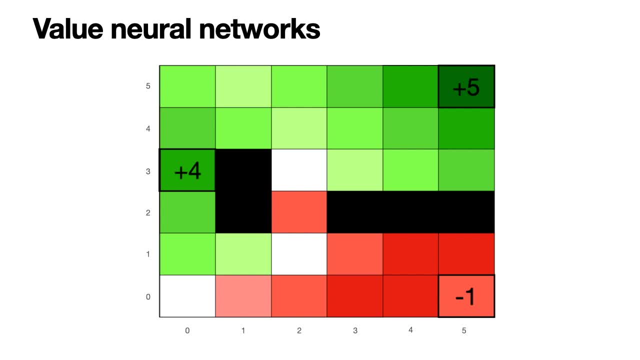 in a neural network that has good approximations for all the values. And finally, once we have this neural network, what do we do with an agent? Well, when we're playing the game, we calculate all the values with the neural network. 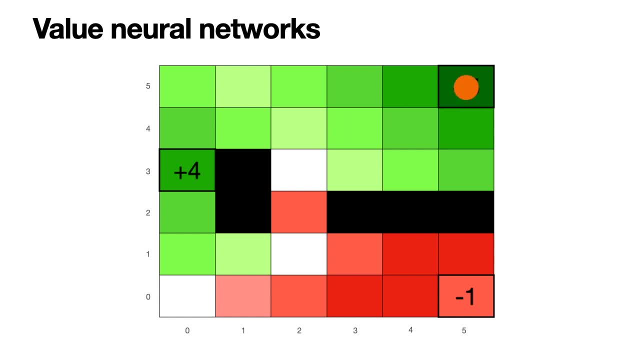 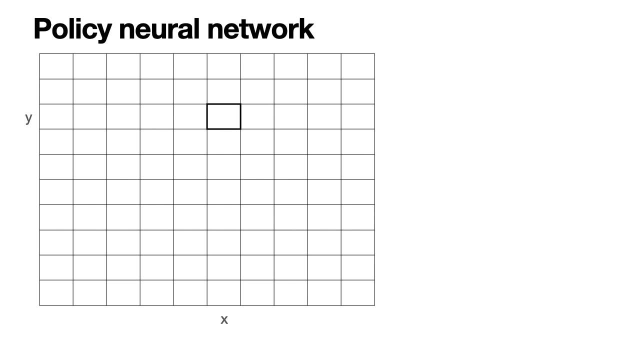 and we simply tell the agent to walk in the direction of the highest value. Now we get to the policy network. In here. what we want to do is train a neural network that takes as input the coordinates of the point corresponding to a state and outputs the policy. 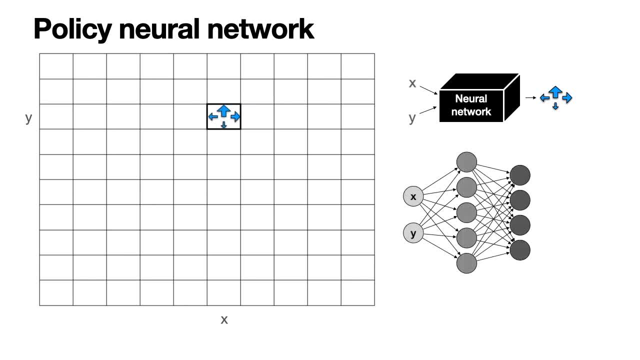 The policy is the probability of going in each of the four cardinal directions. So these are four numbers that must add to one and correspond to the probability of going up, right down and left. Next I'm gonna show you how to train the policy network. 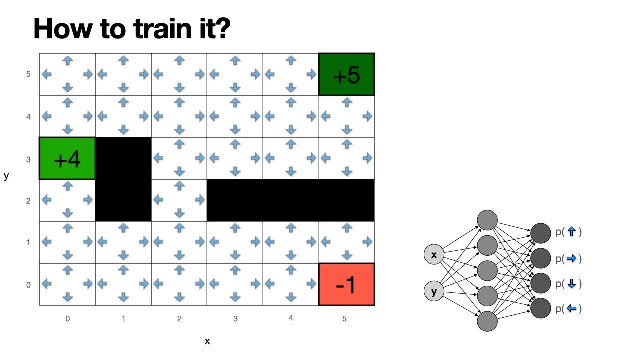 First, imagine that you have a policy network. Imagine that we have initialized the neural network with some weights and it gives us a policy at each point. So this policy has no reason to be optimal because it's just an initialization, which is why we'll improve it. 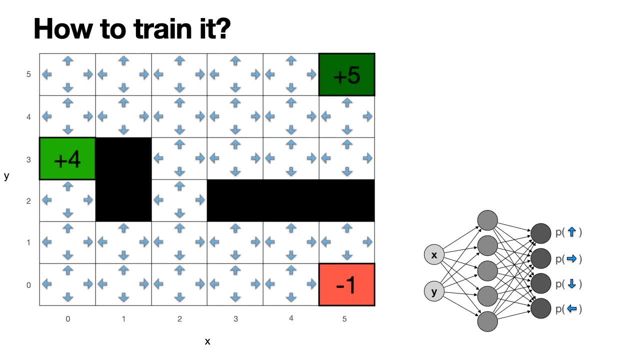 But for now, let's believe the policy and use it to have the agent walk around the grid, where the agent makes decisions on where to go based on the directions that the policy dictates. So let's say the agent takes this path and ends up at the plus four. 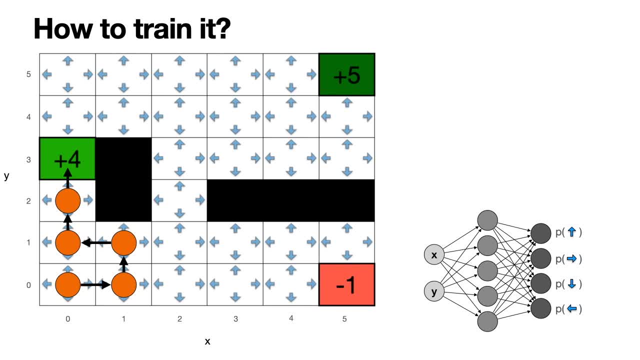 Now, based on this path, and only on this path, what are the values at the states? Well, the state right before the end, since it walked into a four and the reward is minus one. then it gets a three. For the same reason, the previous one gets a two. 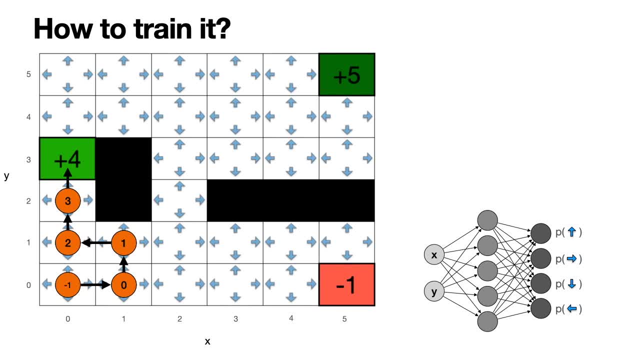 then one, then zero and then minus one. Now pay close attention to the next step, which is the key step. We are going to create a small data set with features and labels based on this path and we're going to feed it to the neural network. 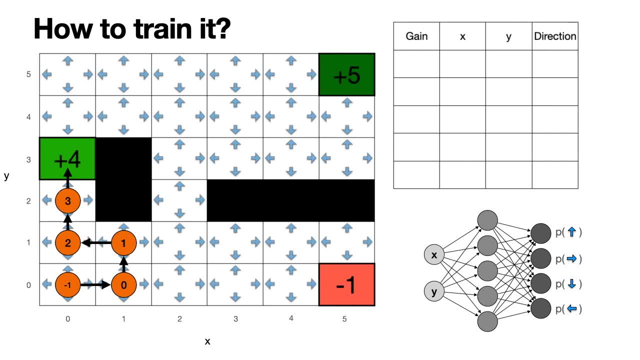 So let's record the coordinates for each point of the path. What we're gonna record is the X coordinate, the Y coordinate, the direction we took and the gain, And we do that for every single point of the path. Now what we want to do is either encourage 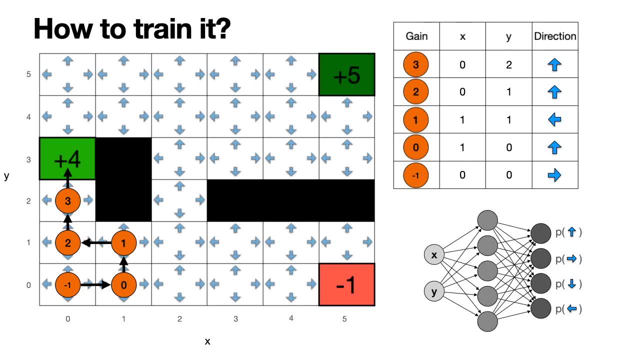 or discourage the neural network to take these actions or these directions at the points of coordinates X and Y, based on the gain, For example, let's look at the top point. At the point with coordinate zero two, the neural network went up, the agent went up. 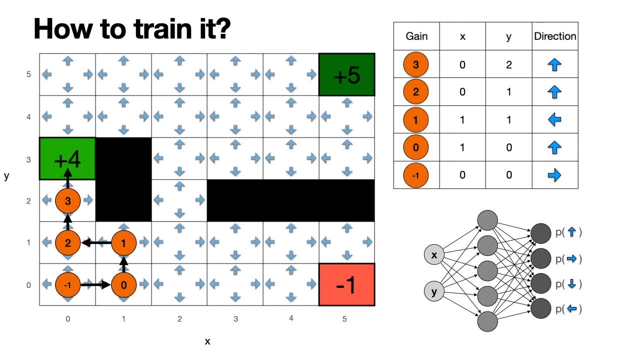 and it gained three. So that's a good move. So we should tell the neural network: you know what, Whenever you reach that point zero two, make that move. So encourage the neural network to take that move For the point with gain two. 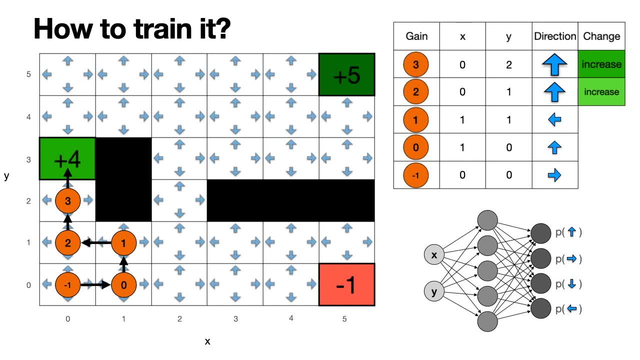 we should also encourage it to take that action, not so much because it was a gain of two instead of three, And for the point with gain one, we should encourage it to take the action at the point one, one to the left, but not as much. 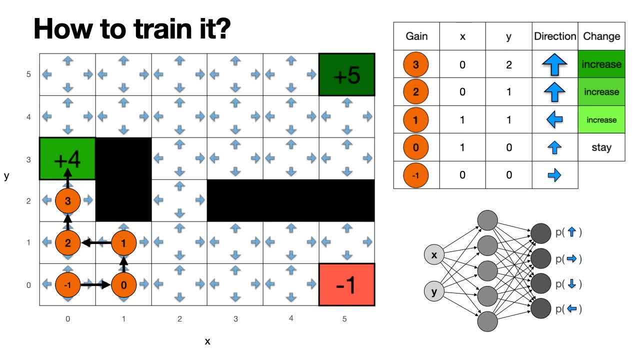 For the point one: zero and the action up. well, it gained zero. So let's tell the network. you know what? Don't worry about that action. And for the action right on the point zero: zero, which is the beginning of the path. 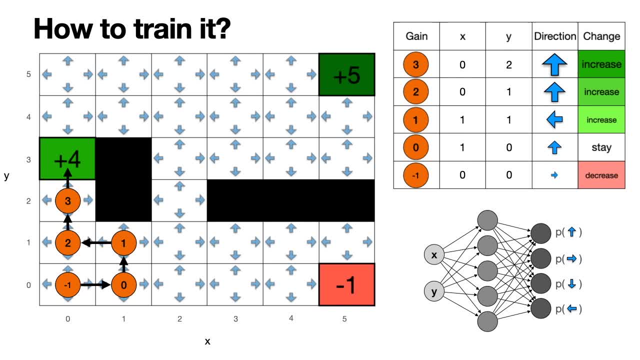 there was actually a loss, a gain of minus one. So we should tell the neural network you know what? That was not a good move. So decrease the probability of outputting that move. And that is the table that we feed to the neural network. 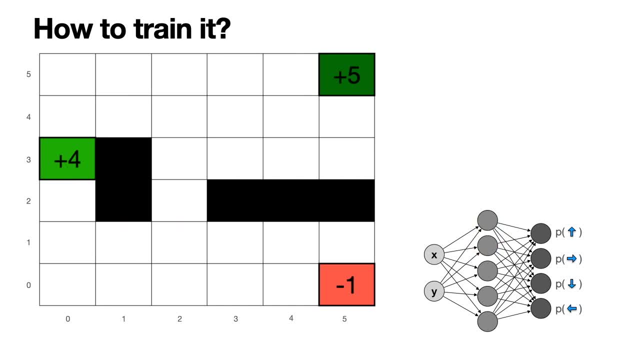 So that is the main step in training a policy gradient. If there was a little confusing, let's do it again. Let's take one path that reaches the plus five. We label everything with the corresponding gain based on the path. So four for the previous one, before five. 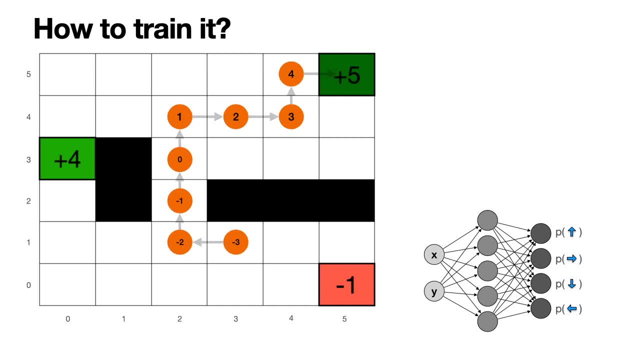 because the reward was minus one and et cetera. And now we're gonna consider all these actions and we're gonna either encourage or discourage the neural network to take these actions in the future. So we create our data set with the gain, the X and Y coordinates and the action taken. 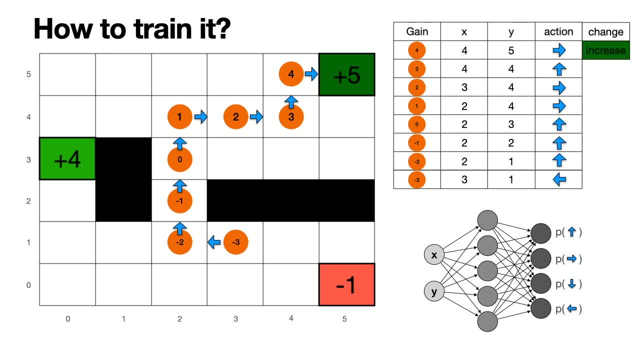 And, based on the gain, we're gonna encourage the neural network to take the steps action go to the right at four, five and all the way to discouraging the neural network to take an action left When it's at the point three. one, 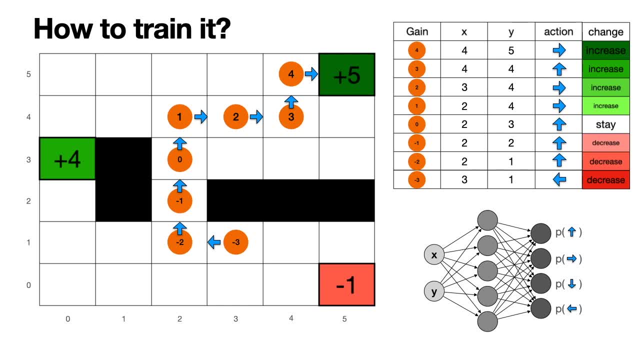 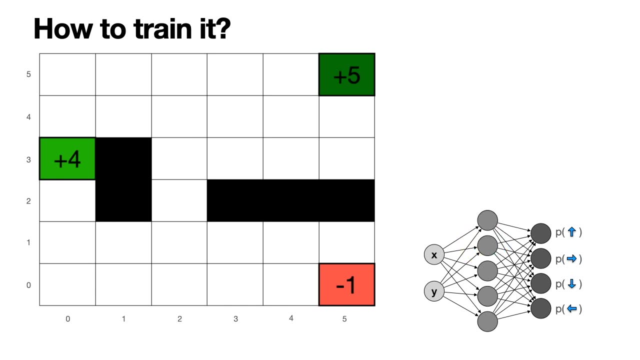 because I resulted in a very bad game. So, in other words, we want some of these actions to be more worthy in the future and some to be less worthy. We feed all this information to the neural network, and that is another step, And we continue doing this. 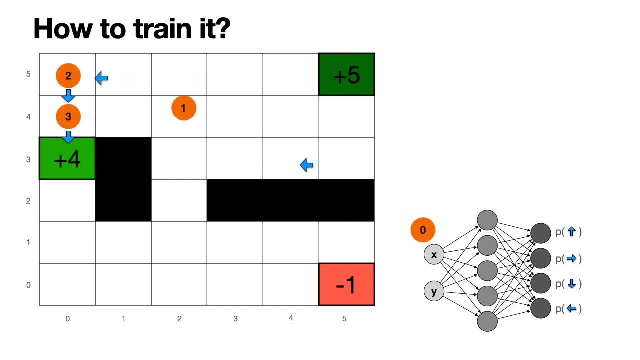 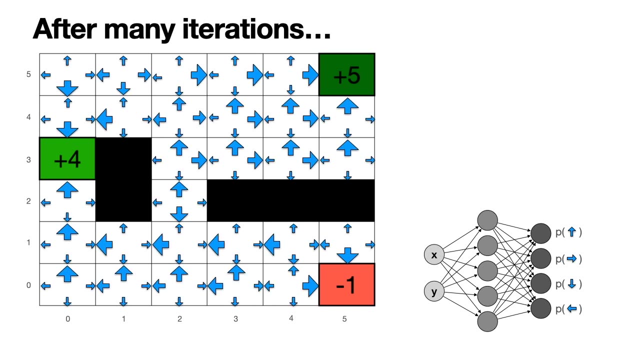 We take a walk based on our policy, we number it and we feed it to the neural network. We take another walk and again we number it for the gain and feed to the neural network. And it's believable that after many iterations, you will be encouraging the good moves. 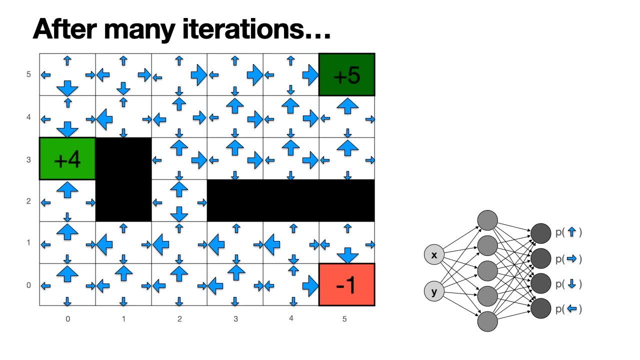 and discouraging the bad moves for every one of the paths, And eventually you will reach some policy that is pretty good. Notice that this policy is stochastic, So it still allows us to walk around- The probabilities are always non-zero, but it points us to the directions of highest risk. 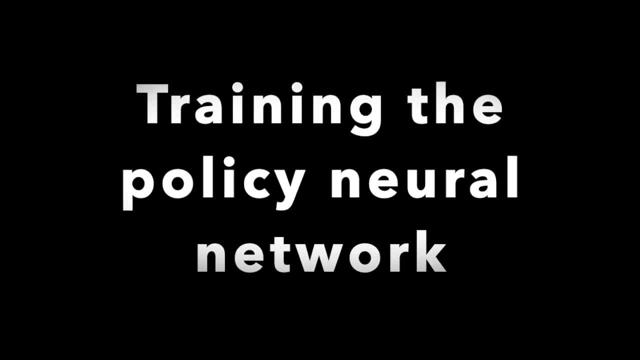 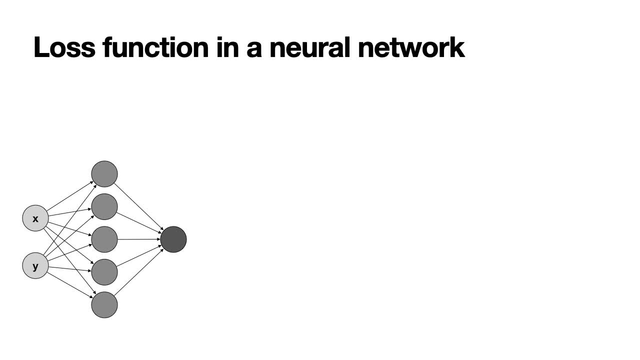 gain all the time. Let me get into a bit more detail when it comes to training the policy network. The way we train a vanilla neural network is by taking a point with features, say 4, 5, and a label of say 1, and what we want to do is try to get the neural network to output as close. 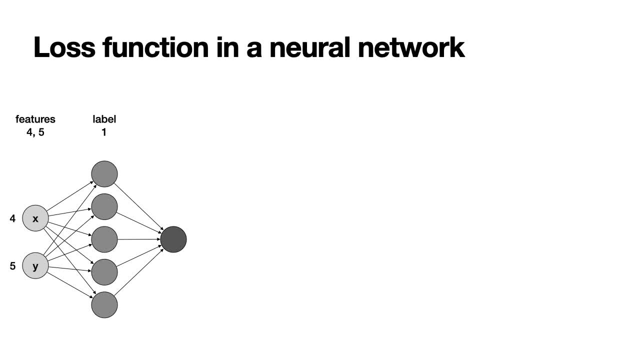 as possible to a 1.. So if the neural network outputs, let's say, a 0.2, that's what we got, which is a probability, and what we wanted was a 1.. So we have to tell the network: hey, network, your task is to increase that answer of 0.2. when I give you 4,, 5 as the input, and actually for reasons, 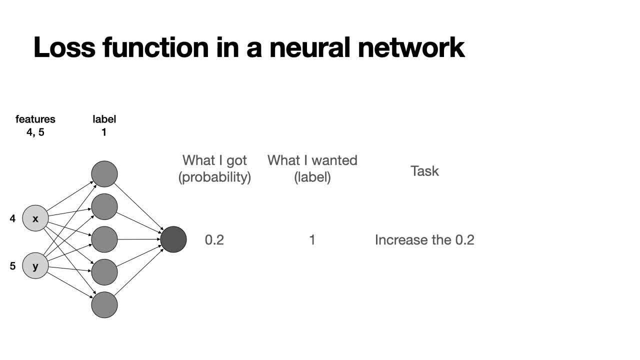 having to do with calculus and probability, maximum likelihood. what we actually tell it to do is to increase the logarithm of 0.2, the natural logarithm, and that is called gradient ascent. You may have seen this gradient descent as well, And the step is to update all the weights of the neural network by adding a learning rate times a. 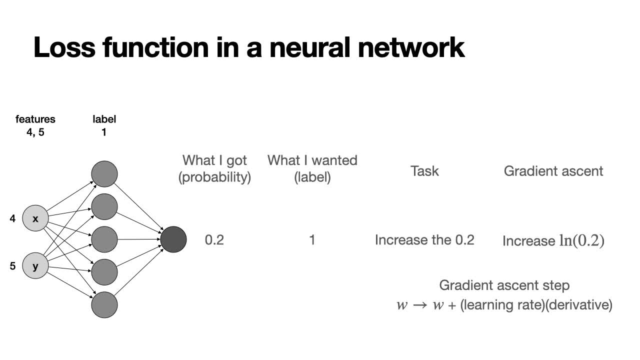 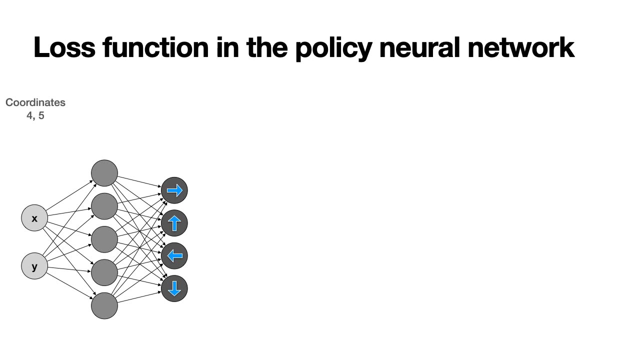 corresponding derivative, That's the derivative of the loss function with respect to that particular weight. So this is what we do in normal neural networks. We're going to do something very similar in the policy neural network, but with a small trick: The coordinates of the points are going to. 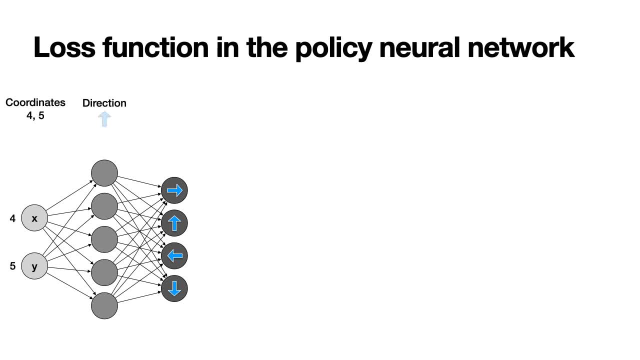 be the features, so they're going to be 4,, 5 and now the label is going to be the direction. So let's say that the policy network outputs a 0.2 for that particular direction and we want it a 1 because let's say that we want to encourage the policy network to output that direction more often. 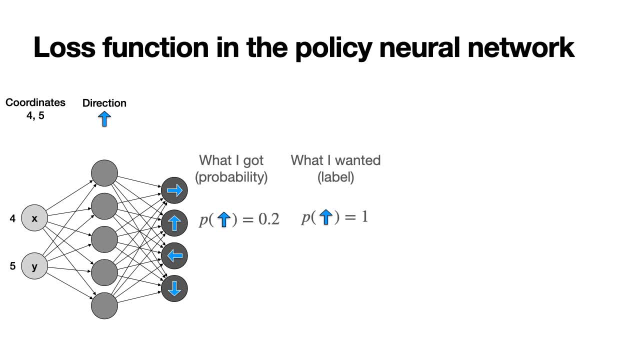 when I give it the input 4, 5.. So what we do is we tell it to increase that 0.2.. Now, again, for gradient descent reasons, what we want it is to increase the logarithm of 0.2.. But now remember. 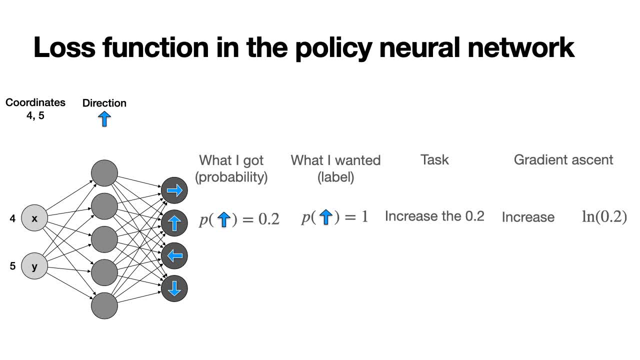 that we want the neural network to increase the probability of all the actions, only the ones that have high gain. So if the gain is, for example, 4, what we do is we cheat this error function and we multiply it by 4.. So now our gradient descent step. instead of updating the weight by the learning 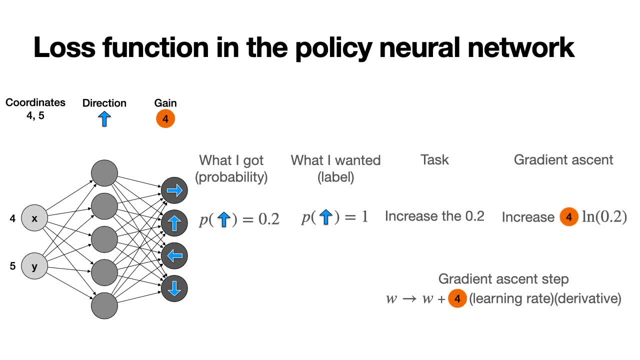 rate and the derivative for each of the parameters of the neural network. it updates it by the learning rate times, the derivative times, the gain. So what happens, for example, if the gain is negative? If the gain is negative, we want it to discourage of taking this action and so we multiply it here and we actually the neural network goes in the. 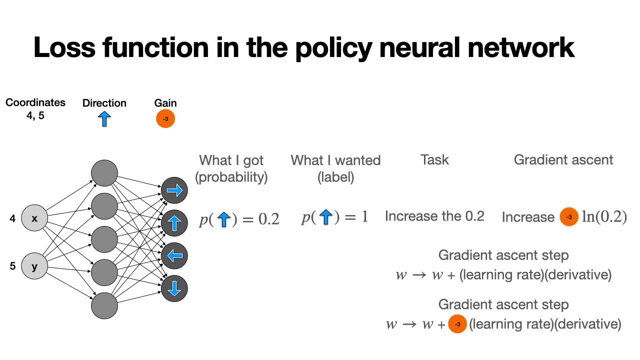 opposite direction, thus discouraging that direction to happen. So that is, in large scale, what we're doing. We're tricking the error function by multiplying it by the gain, so that the policy network will be encouraged to take steps with high gain and discouraged to take. 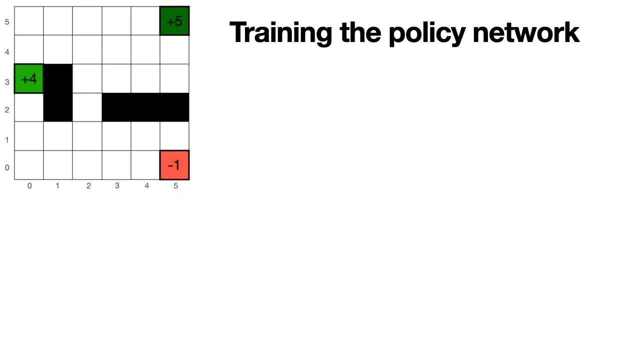 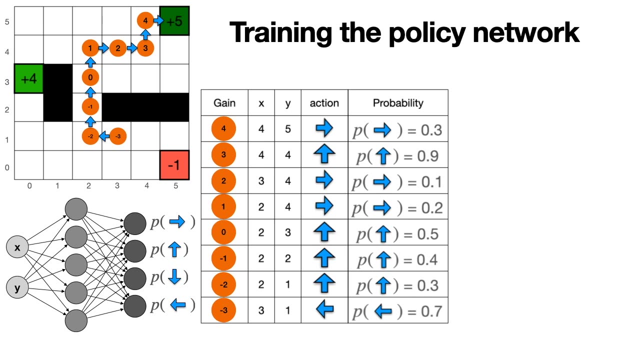 steps with low gain. So that's pretty much it. At every step, you take a path and what you want to do is make a small data set where you have the features, the action and the gain. the features are the coordinates. These are, let's say, the probabilities that the neural network give you from the beginning and you 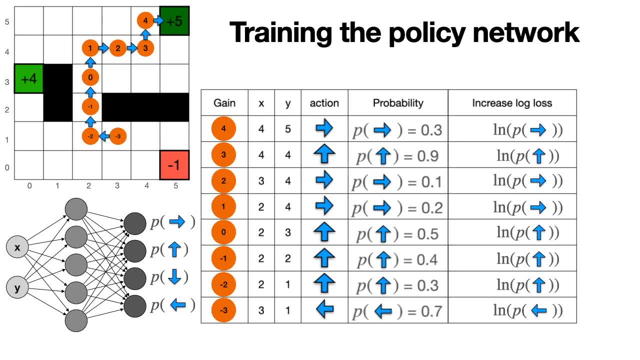 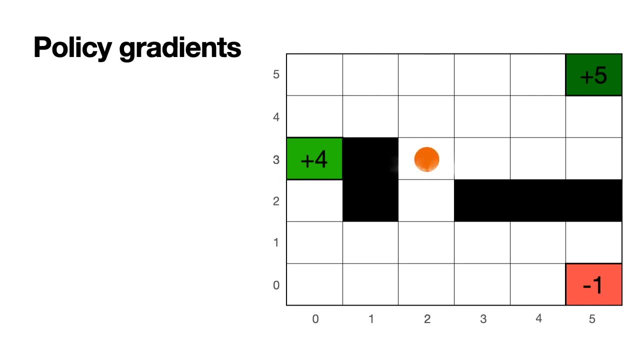 want to increase these logarithm, but multiplied by the gain And that will tell you which steps you want to encourage the neural network to take more and which ones you want to discourage the neural network to take. And that's pretty much it. Once you have your network trained, then when your agent is here, you use the. 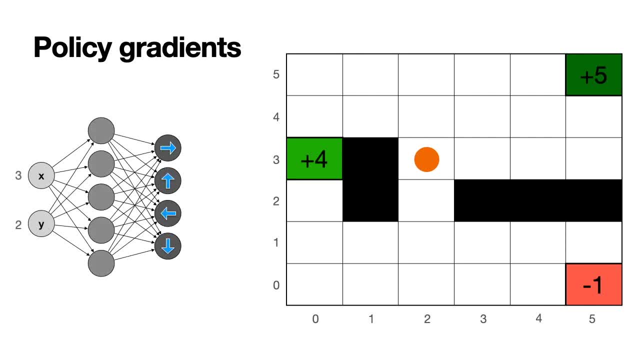 neural network to come up with the policy at each point and you use that policy to move around. You would normally take the step with highest probability, but you take a step with the probabilities given by the policy And you, with high likelihood, you end up moving towards the points of high value. 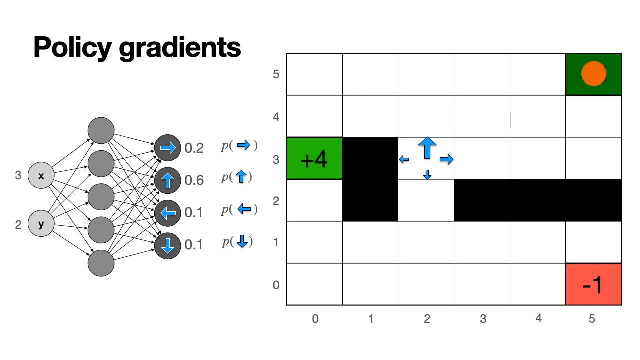 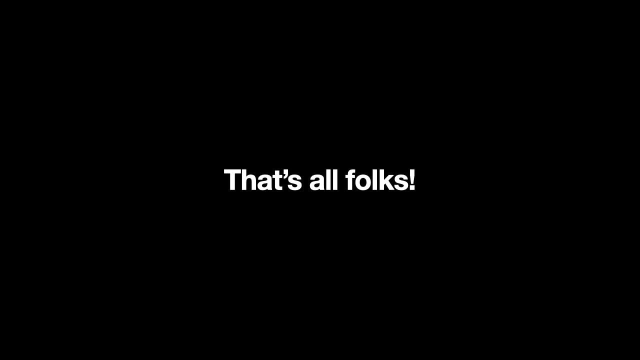 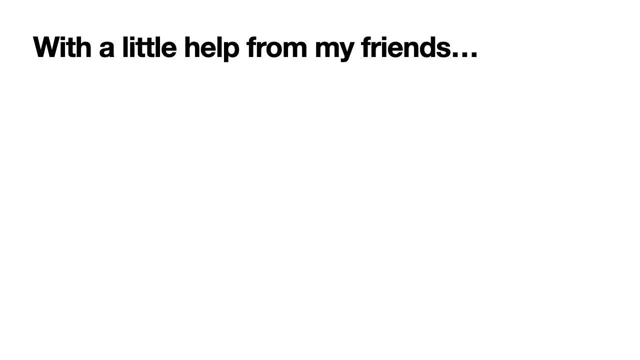 But you are always able to explore the space. And that is all, folks. Thank you very much for your attention. That is how deep reinforcement learning works. I hope you enjoyed this video. I would like to thank my friends, who are very, very helpful, and I wouldn't have been able to do this. 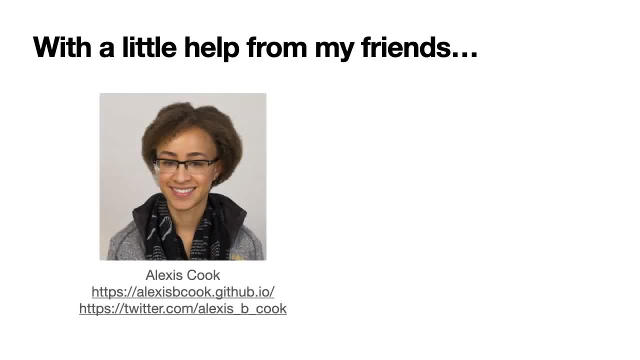 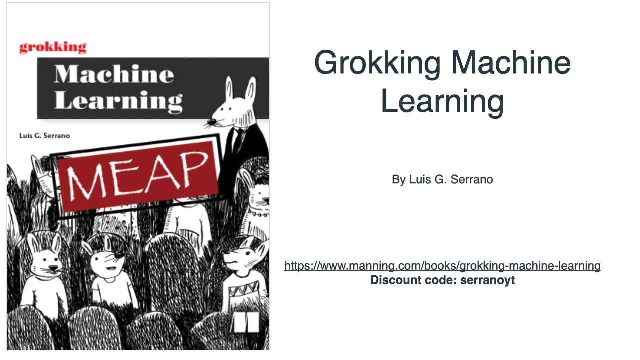 without them. There is my friend Alexis Cook, who is an expert in deep reinforcement learning- It was very helpful- And my friend Christian Picon, an expert in machine learning, and helped me with the material and also with some code. I'd like to remind you that I have a book called Grokking Machine Learning, where I talk about the